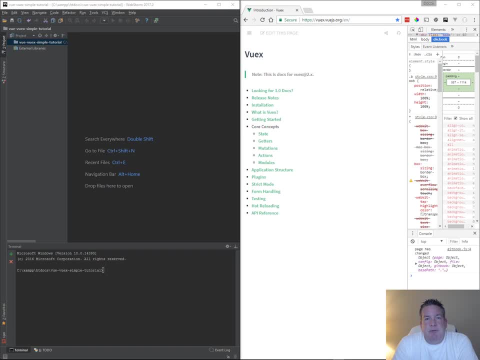 Okay, today we're going to talk about implementing VueX and Vue in the same basic project. One of the things I've noticed, especially with myself, is that I kind of was hesitant to get into VueX because really I enjoy programming in Vue and I needed to learn how information traverses from component to component. So, you know, we had a main component, we put a component in it, we'd use props to come down into the component, we admit events back up to the main component, and if that component needed to talk to a sibling, you know, we would then have a method on the main component and then, you know, handle that through a prop down through the second component and then, you know, event back up. That's really, you know, important in the learning aspect of it, but as far as trying to get some big production, that's really not efficient and can get really messy and as your program gets, your application gets larger and larger, well, that's the, it's going to be almost impossible to maintain. 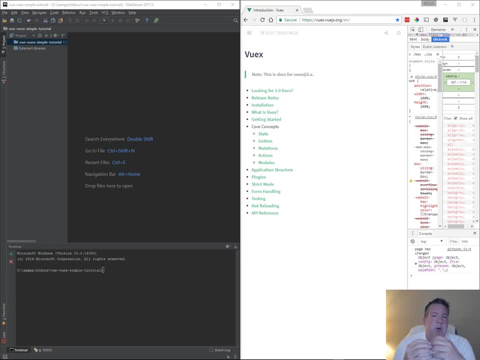 So what we have is we have VueX as our state management system and it's so easy to put into the system, unlike in React and the multiple state management systems that React had, whether it be Mobex or, you know, Redux, Redo, however you want to say it. 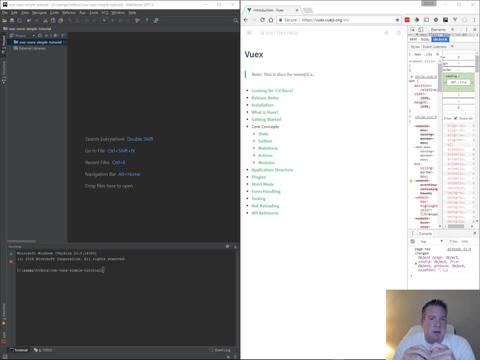 They were, you know, because they started off with the Flux thought process, you know, I didn't really understand Flux. It was not a, you know, it's not a piece of software. It was a, it was an idea and I didn't have the knowledge at the time to, you know, be able to do that. To, you know, try and, you know, begin to understand that type of modularity. Of course, now we're a little farther along and modularity is everywhere. Webpack is a required tool almost in, in JavaScript front end programming. Obviously, it's not absolutely required. We can still script out longhand inside the, inside the page and for certain applications, I'm assuming that's, that's absolutely fine. But, you know, it's not absolutely necessary. 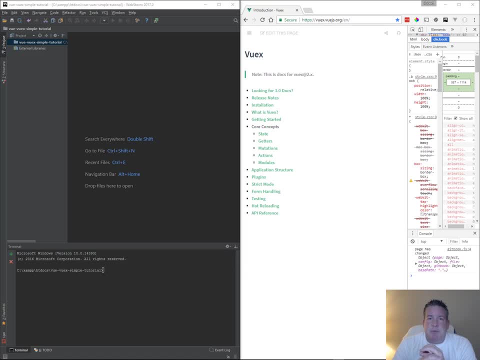 almost, in JavaScript front end programming. Obviously, it's not absolutely required. 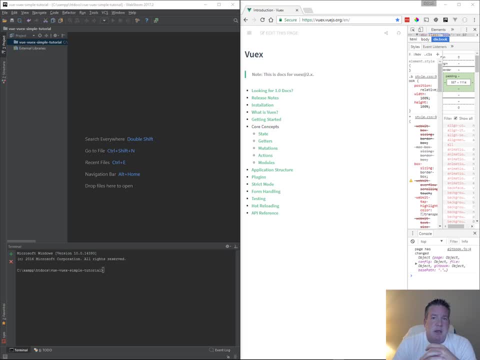 We can still script out longhand inside the page. 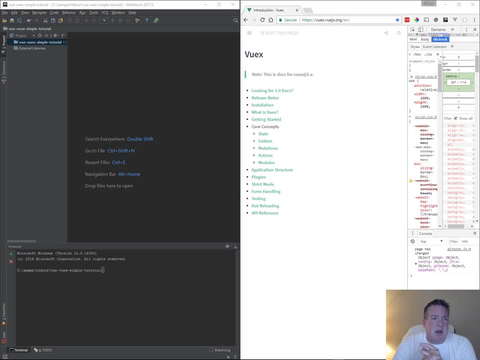 And for certain applications, I'm assuming that's absolutely fine. I don't do that anymore. I used to. I loved it with Angular 1. That was my introduction into these framework systems. And it was fun, and it was quick to create stuff. 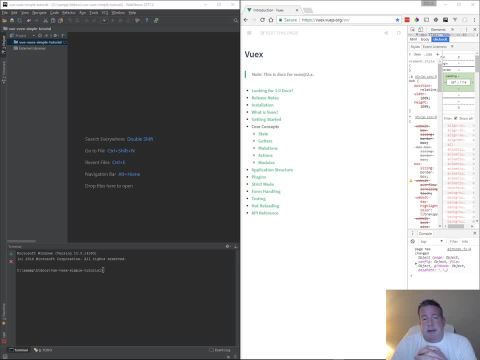 And then Angular 1 turned into Angular 2, and I didn't like it. 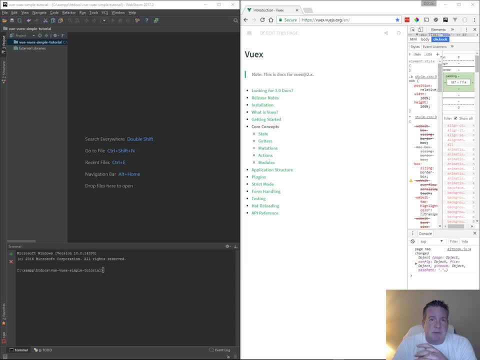 So I went over to React, and I loved React as far as the component construction. And once I learned how we did the propagation of information through props and, of course, events, which is the same way that Vue does it, that became really fun, except that I didn't have state management like I did in Vue. 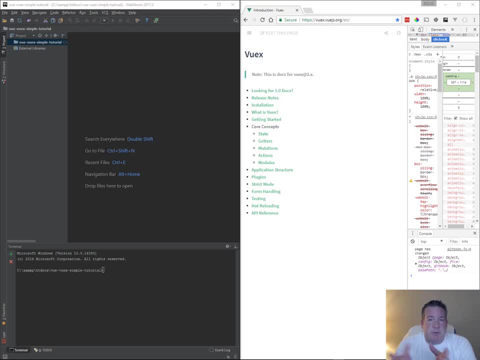 Angular 1, of course, Vue now merges those systems, has state management both at the component level, above the component level, and, of course, in its total store system, its version of Flux. 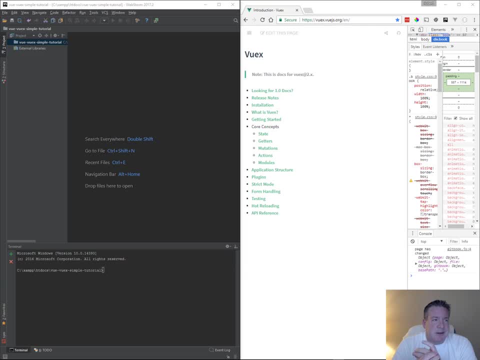 But I wanted to show you how easy it is to both create a project and that you should just dump the store in it almost every time you create it. 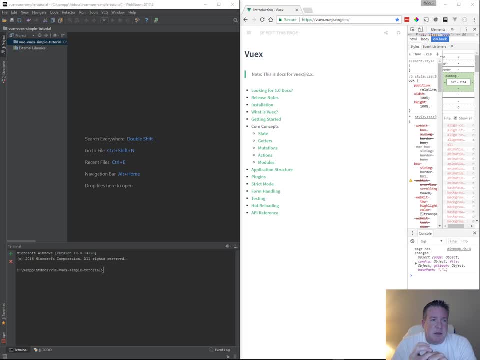 I would actually prefer that they did that in the skeleton, scaffolding of the system when they bring in the CLI. 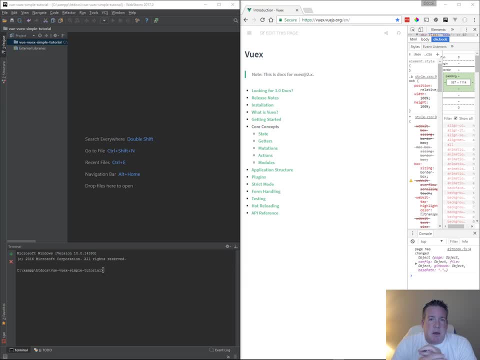 It's just to ask you if you want Flux. It's part of the primary program. 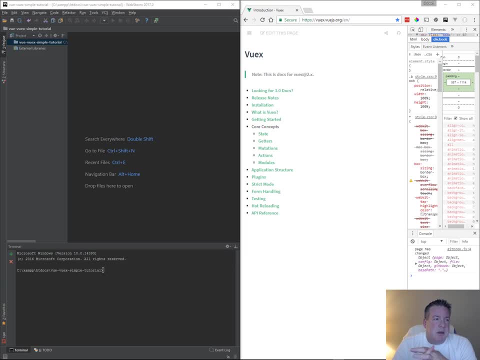 It's not a third party program, per se, like Redux or MobX or anything like that. 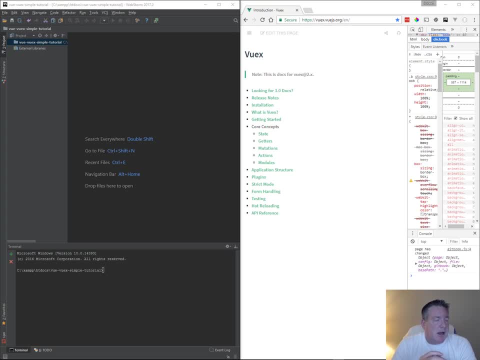 It's built by the same person, people. And I just think it should be part of the system. And just go ahead and scaffold it out for you. There's no reason not to. But let's go ahead and do it real quick. I mean, it takes literally three minutes, if I'm not talking, to do. So let's go ahead and just initiate a new Vue program. I'm using WebStorm. So I've already started a new project. 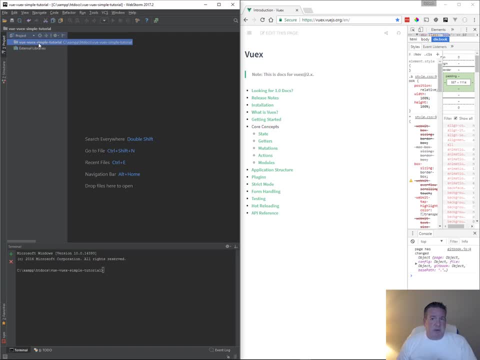 It really is as simple as doing the file, new project, naming it. 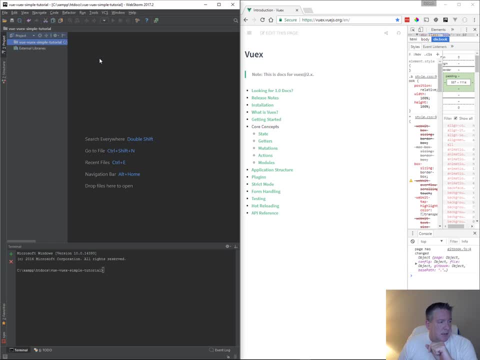 I don't have anything in the background or anything to hide something that you may need to know to get us going. So WebStorm has a built-in terminal that obviously grabs the Windows terminal, in this case Windows. So one of the reasons I really like WebStorm and PhpStorm is the fact that they really kind of just pack everything into one. I don't know. 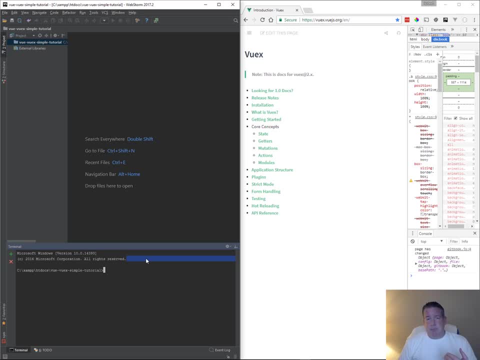 I don't know if you're familiar with WebStorm, but WebStorm is an IDE. And it really is integrated, whether I'm doing my NPM, Node Package Manager, or modular system. And I want that brought out in scripts to the terminal, to the database. It will pack individual files. So if you are a scripter, a person who puts the script directly into the page, you can have WebStorm.com. I don't know. I don't know. WebStorm can minimize those for you and put them in min files and obviously babble down the 2015 and the ES6. 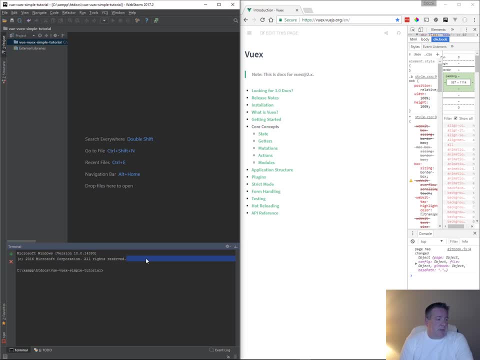 So it's a great program. Both of them are. I love them. They're very convenient. 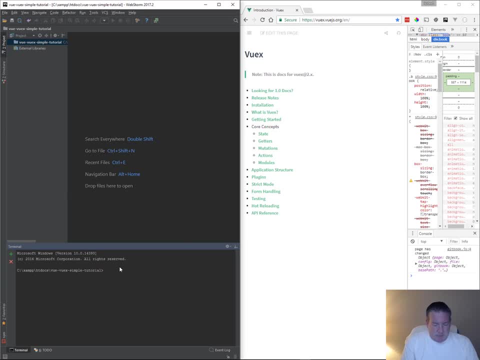 But anyway, so we're going to go into our terminal. And we're going to do, let's do view init Webpack. And we're going to do that. 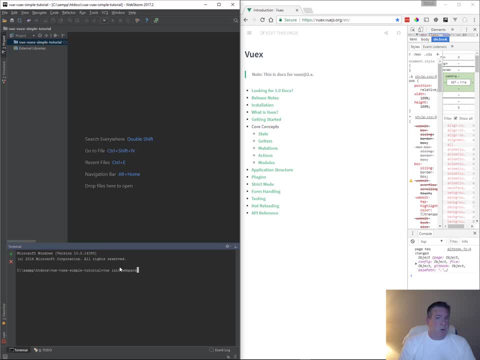 And in this particular case, because I've already started a project, I've already created the folder that it's going to be in. 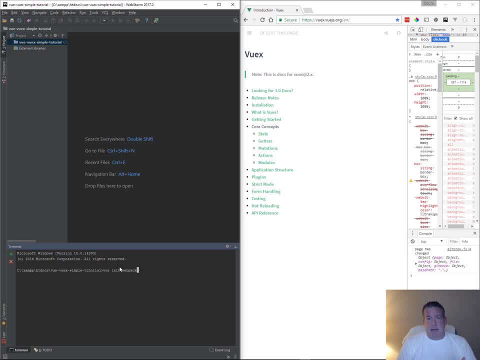 I'm just going to leave this blank. So if you do view init Webpack and leave off the package name, it will ask you if you want to do it in the same folder that you're already in. And I'm going to say yes. If you are using a straight terminal, obviously you need to add the folder name or the package name, both synonymous. And it will create that for you. And of course, you'd have to change directories and go into it. But I'm already in the directory I want to be in. So I'm just going to hit enter. 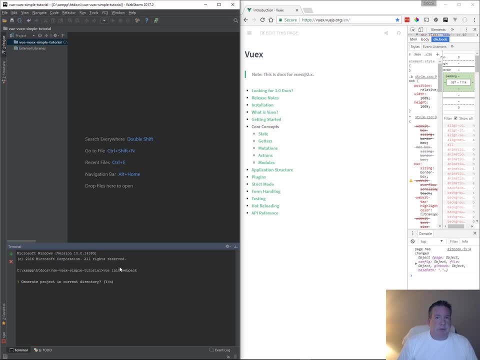 First thing it's going to ask me is if I want to create the project in the folder that I'm in. And the answer is yes. 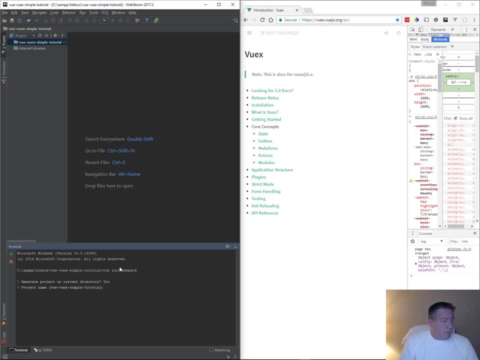 So then we've got the project name. We've got the project description. We've got the author. All of them defaulted on my system. I'm sure they're going to be defaulted to you. They don't. They certainly don't matter in the tutorial. 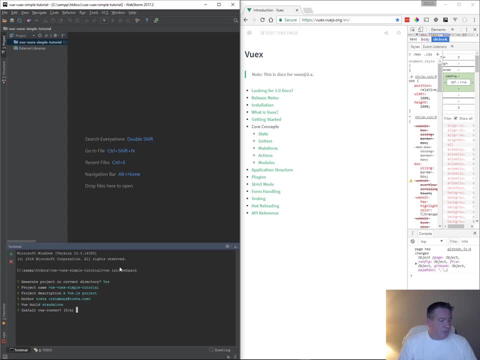 Runtime and compiler. I'm going to go ahead and install both of those because I don't want any problems with hot reloading. 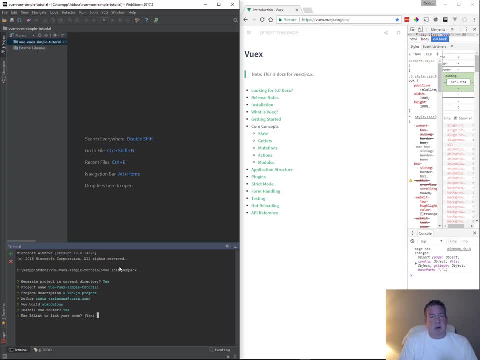 I always install the view router. Always install the view router. It's just something I don't want to do later, ever. So even if I'm doing templates and I know I'm not going to use it, I'm going to install the view router. 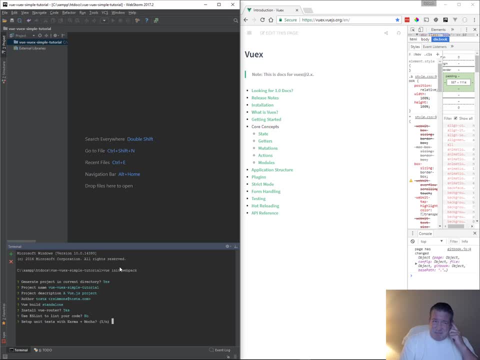 ESLint I do not because I have problems with semicolons. So my semicolons typically don't end up in the right spot for ESLint to like them. And that's just old school. 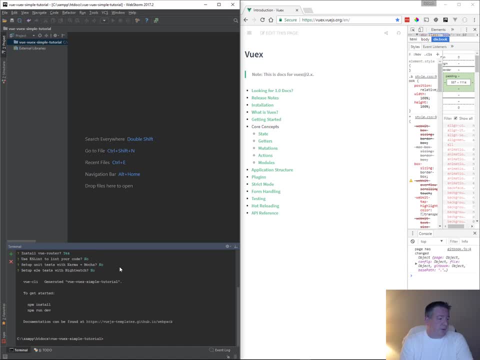 All right, and we're going to do no testing on this, obviously. All right. So now we've got our scaffolding done. 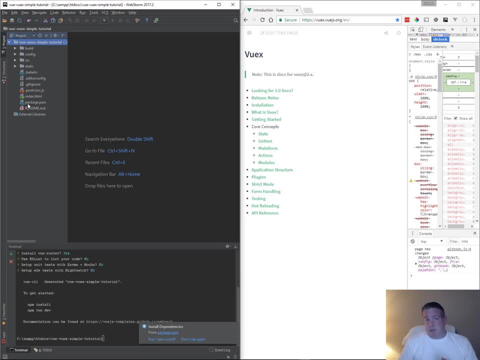 We can look here and we can see the scaffolding. There's no node modules in here. So we need to obviously run the npm install to go ahead and bring in our dependencies. 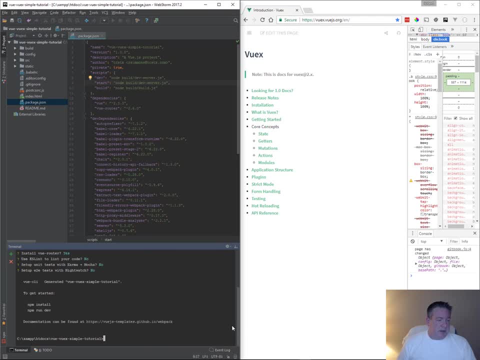 So and of course, it's asking us if we want to run that. I'm just going to shut that down so we can do it by hand, npm install. And we're done. All right. All right. All right. 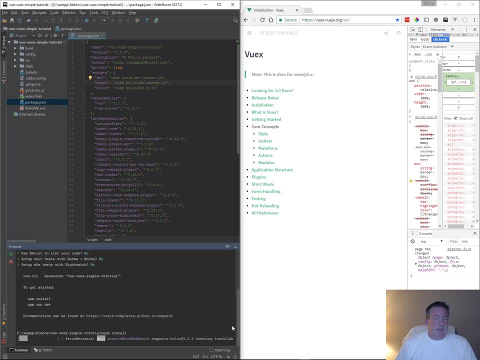 And while that's installing, we've got a nice old trick that WebStorm and PHPStorm allow us to do, which is to abstract the scripts out of a package.json file and put them into the GUI, into the GUI, so that you don't have to type it every time. 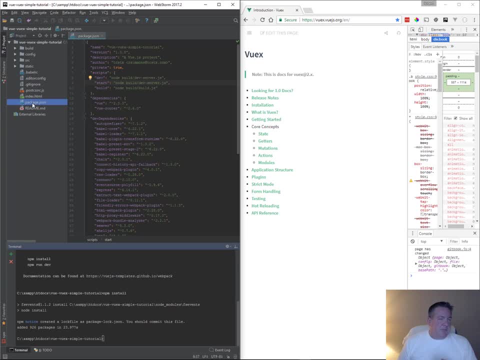 Some of them are self-starting, but some of them can be long, especially if you're doing long scripts. 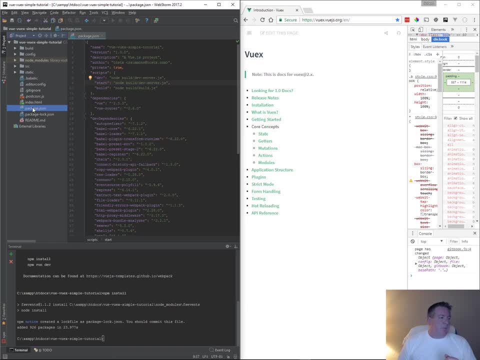 These are pretty short, but I don't want to type them out. So we can just go to our package.json file and show our scripts. 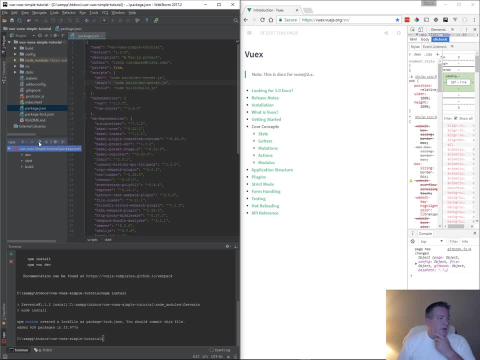 So give it a second and populate here, do a refresh. There we go. And it's just populating the scripts here from our package.json file. 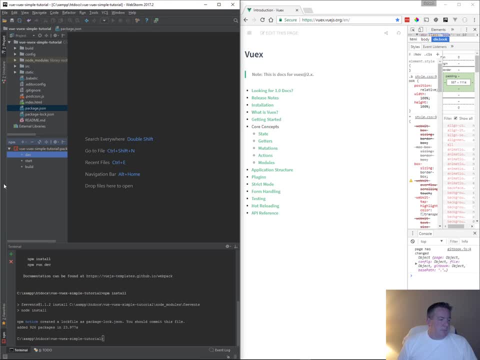 Now we have a completely running Vue program application. I'm going to go ahead and just CLS this out. All right. 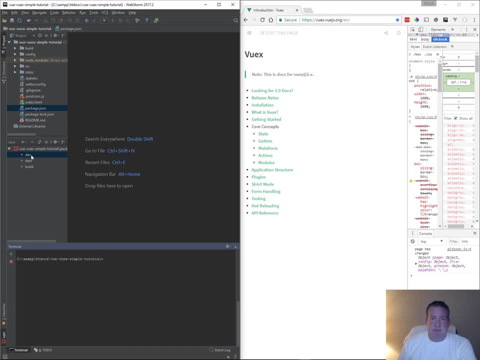 And the easiest way to start it is just double-click on our dev. If you're running in a terminal and you're not using PHPStorm or WebStorm, you can just 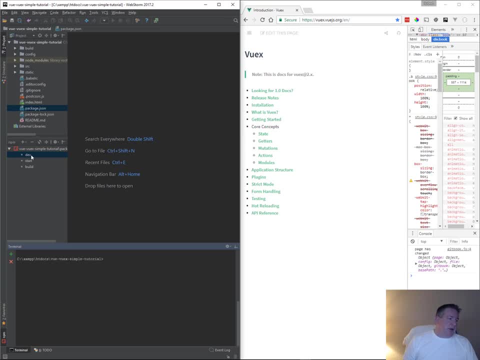 type npm run dev, three words, npm run dev. 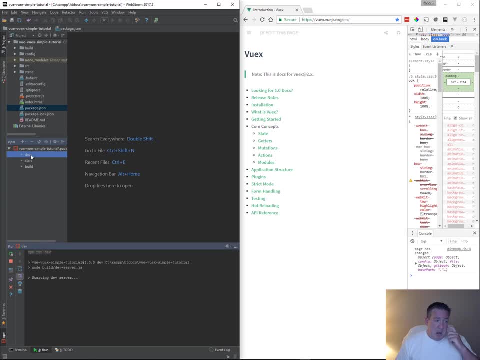 I'm assuming you already know this because we're doing a Vuex tutorial. Okay. 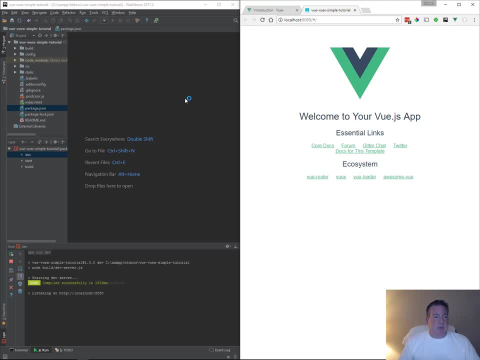 So we've got Vue installed, no Vuex, but we've got Vue installed. It's a completely running application. All right. 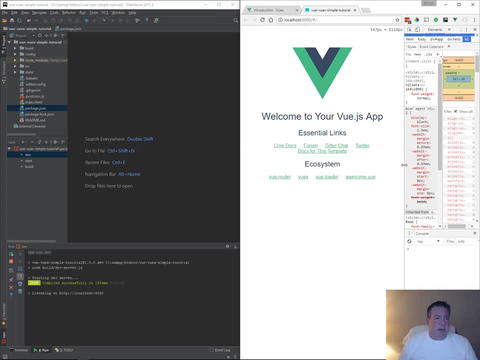 It's running a router. I'm going to turn on the inspector real quick because we don't want it caching. And as you can see, there's no problems or anything, even though it may show up that it's missing a favicon or something like that. But it's a completely running application, but we don't have any outside state management. And if all you're doing is building a component, then you don't need the store, obviously. But if you're going anywhere beyond that, then... Having a store is just better do it now, eat the frog as it were, and go ahead and get it done. That way, you're not building something you get tunnel visioned in and you start writing a bunch of props and events to handle something that the store really should be. And then once you go back to move all that or moving that into the store, then it becomes, well, difficult. Because it's hard to follow, sometimes, props that create events that emit up to the primary that may have just something else. That's the whole reason state management and the store system was developed is because it's difficult to try and follow some of those. And when you have a bug or just moving them to a different area or renaming them can be just a spaghetti system gone wild. Anyway. 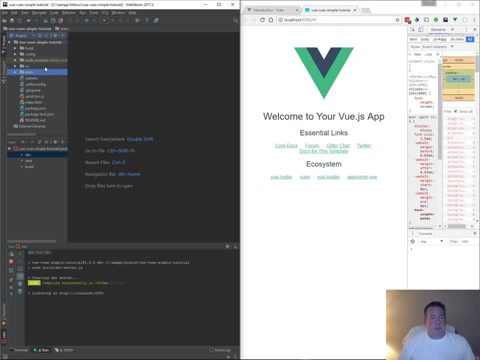 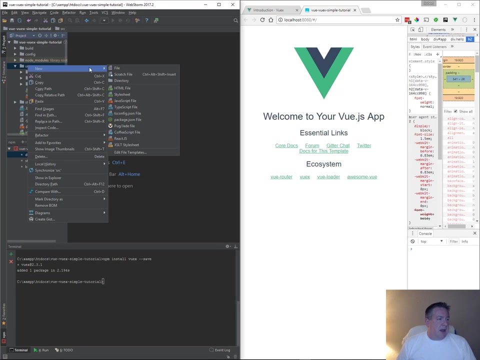 So we've got our basic system and the first thing we're going to want to do now is go ahead and add Vuex. So we're going to bring up our terminal right here and npm install Vuex and we're going to save that to the package manager. Because it's part of the primary program, we're doing save instead of save dev. All right, it's all done. So to utilize that, we're going to go into our source system. And we're going to add a file and it's just going to be store.js. 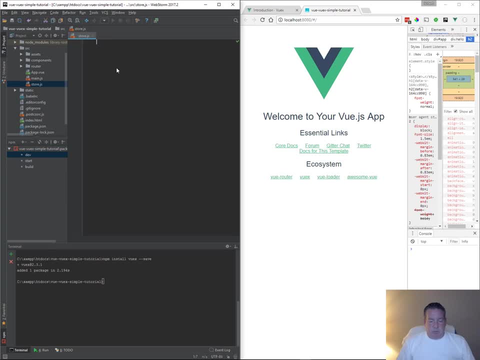 And from here, we're going to go ahead and bring in Vuex. So we'll just start with import Vue from Vue. 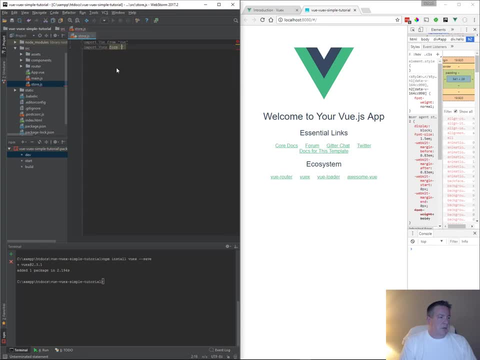 And import Vuex from Vue.js. All right. 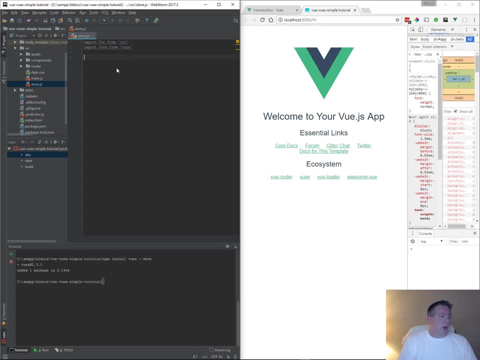 We're going to put it into the Vue, implement it into the Vue system. So we're going to do Vue.use Vuex. That's one of those lint problems right there. Doesn't like that. And WebStorm and PhpStorm want it. 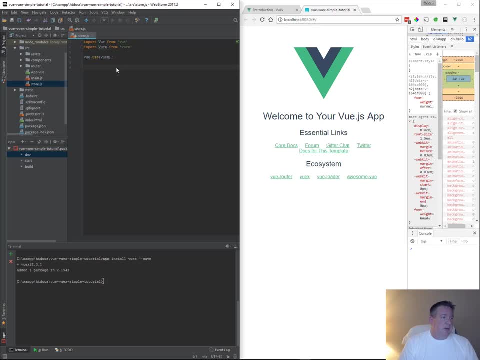 So it's easier for me to get rid of lint than it is for me to fight my IDE sometimes. All right. 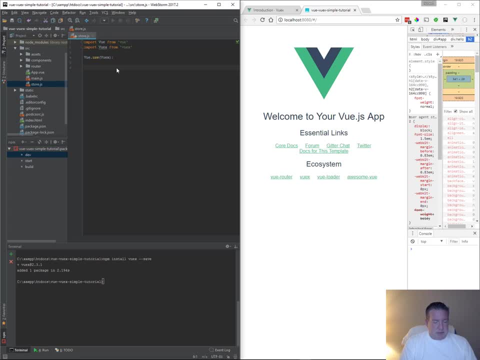 So now we're going to create the component. So we're going to export a component. It's going to be a constant. We're going to call it store. It's going to equal a new object, a new class of Vuex.store, which is the constructor of it. And there we go. 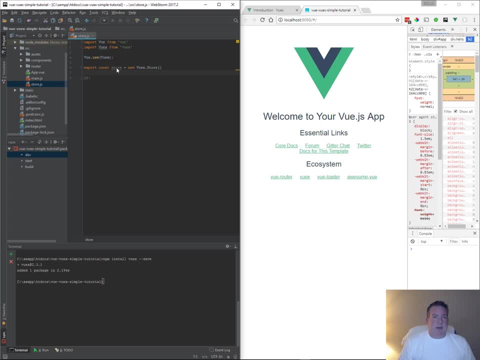 We've got our new class created. 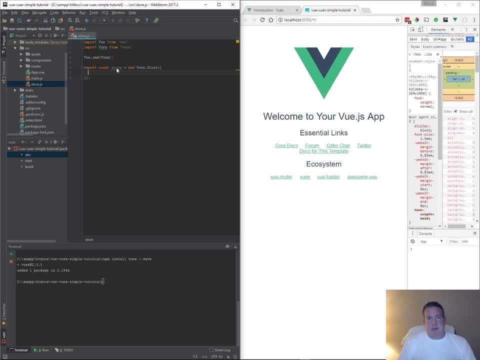 And here we have our one Vue. express. It should probably be the default thing in theaving. It's going to be a regular component. You get athing to every Vuex import function. But what he's going to need is a state. And again, UseVuex is going to be the multi Terminal package. It's free. That's good. 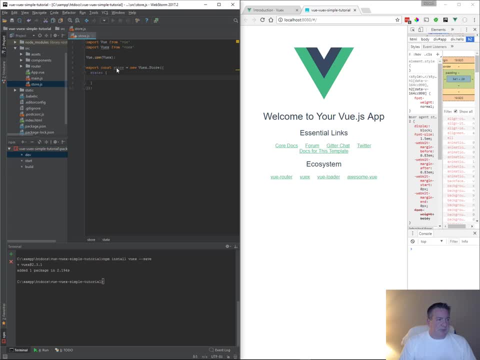 is and mutate the variables in the state but it's not recommended and there's a number of reasons why not only future modularity and expansion and readability but also because you're mutating the the store state and you bypass all of the functionality of time travel and some of the protections that you get from having kind of getters and setters within the system and if you don't know what time travel is in the store system you can look at that if you have the view extension installed in Chrome which I'm you should right there then you can always look at the store right here of course we don't have a store because we haven't implemented into our main app even though we have it abstractly to the side but if you don't have the view extension definitely put that into your your chrome developer browser and I'll show you how that works in a few so we start with state and we need four items we need state we need getters we need mutations and we need actions and that will complete our store it will be a fully functional and properly scaffolded store 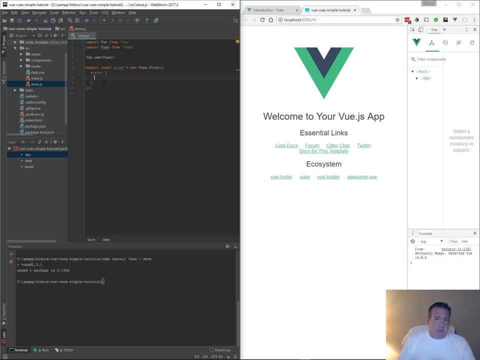 so but I'm gonna go ahead and as we scaffolded out I'm gonna go ahead and add some some but just a pretend one event system so if so let's say just say we're going to put in a variable like is true and we're going to name that but the colon not selection true we're going to start it off right there true and we're dealing with an object so that was a no successful and then the next thing we're going to do is put in together you know I'll show you that So everything is of course named plural in your object scaffolding. So getters, mutations, state, it's not states because that's not really proper. It would be the state, getters, mutations, and actions. 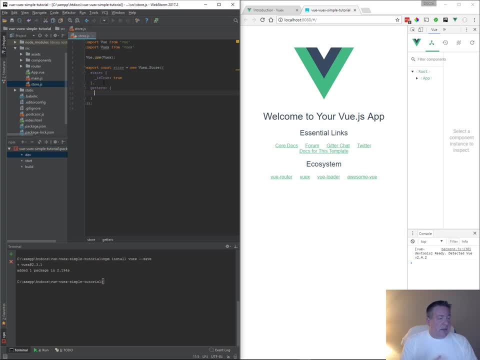 All right, so we've got getters. And in this particular case, let's say that we're going to get something, we're going to get the state of is true. So to do that, we're going to have to have a function. So we do is true, and it's not the same variable, because we don't want to touch the original variable now. The only place we want to touch that is in other functions, so that we don't actually mutate the original variable. So we do is true, and like I said, it's a function, and I'm going to write these longhand for right now instead of using ES15 function. We're going to import state, and obviously if you know ES15 or if you want to do ES6, you're more than welcome to. It's much easier for you to do that than it is for somebody who doesn't understand ES6 or ES2. So we'll do that, and then what we'll do is we'll return our state value. And that way, so if somebody calls it from outside, which they would be doing, they'd call it from outside as a getter, and they'd wonder what is true is, and what it's going to do is it's going to return the state of our store, and it's going to return that variable. And I'm using the... 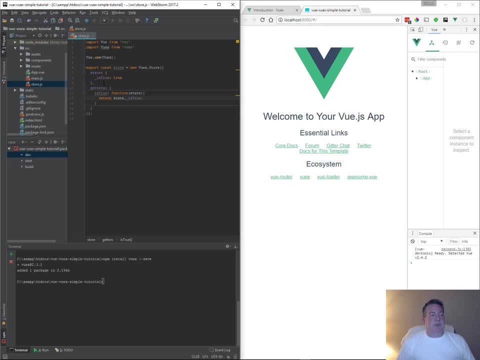 Underscore for no other reason than the fact that it lets me know that that variable is one of my internal variables, and it should never leave, and it should never be used as an input and output system. 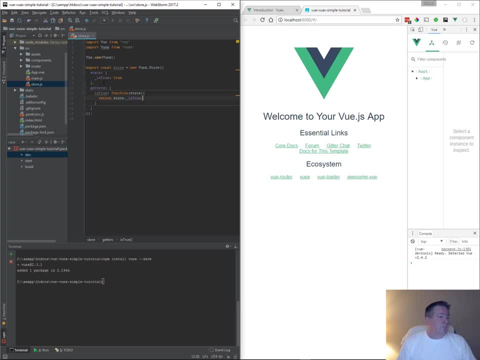 It's the mutatable variable within the store, and it stays in the store. You can use that. You don't have to. It's whatever's comfortable for you. 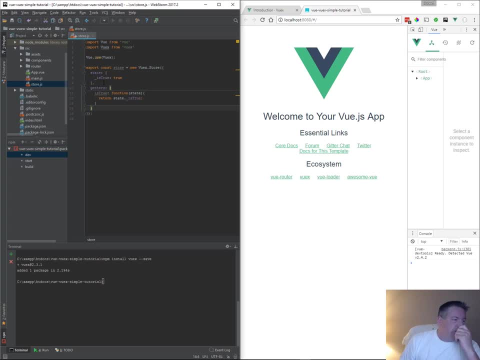 In that particular case, it's comfortable for me. So we've got our state. We've got our getters. 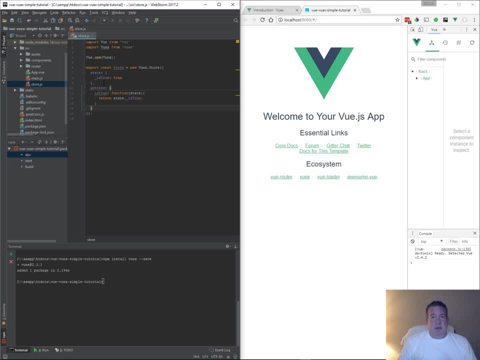 And now we need... To be able to mutate the object. 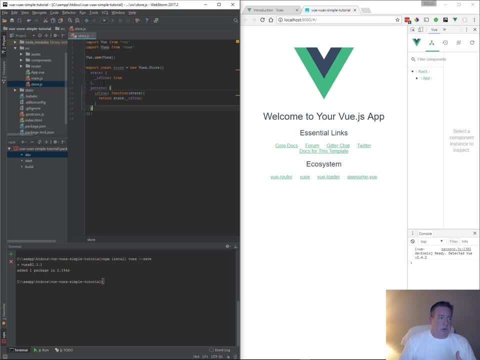 In other words, how do we turn is true to false, or toggle it back and forth? So we need a setter or a mutator. 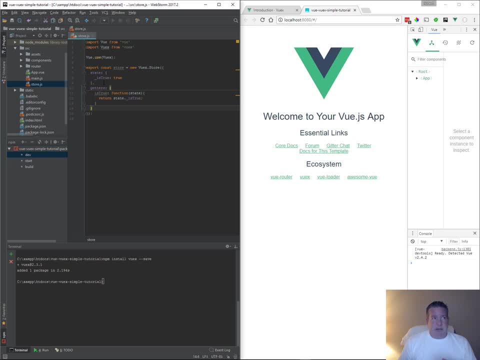 And mutations is actually a better word than a setter, because in object-oriented programming, we use the terms getters and setters. But our setters really did that a lot of validation, and sometimes they mutated the source and, excuse me, mutated the local variables. Like, is true. And so setters wasn't necessarily the right term at the time. So mutations actually ends up being a better word, and we just... Us old school people have to learn that. So we do mutations next. All right. 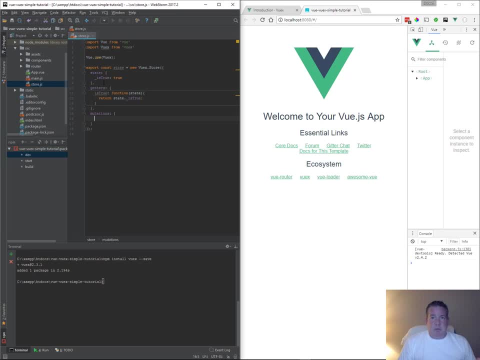 And we're going to want to mutate the original... The original... The original... Object variable. 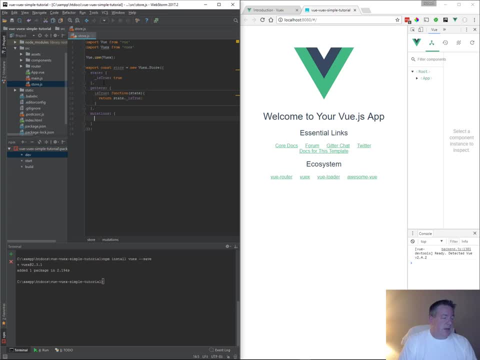 So what we're going to do is... Let's use something like toggle. Because we're going to toggle the state from true to false. Toggle. 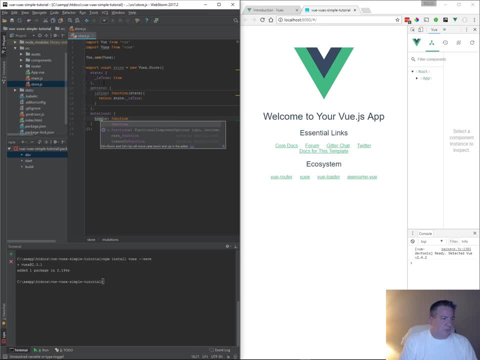 And it's, again, going to be a function. These are all going to be functions from here at pass state. 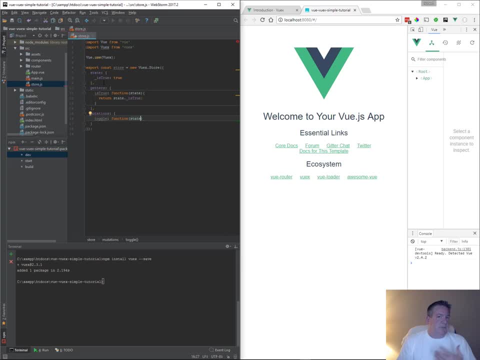 We're going to pass in state. If we wanted to create a function that... 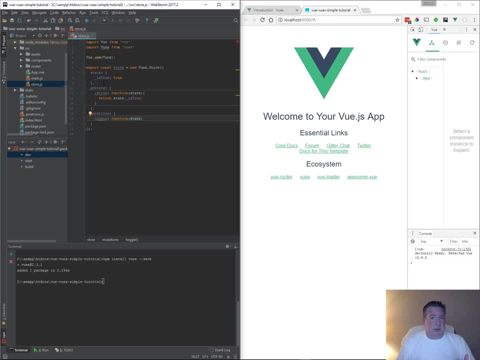 A mutation that had a... Had props, had arguments, you just add them after you add state. So you just add the arguments that you would need to operate on your variables or perform what you need to do. 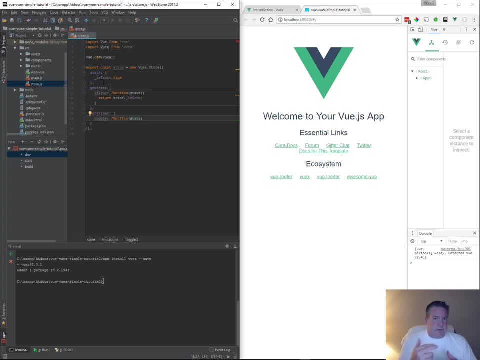 And you'll do the same thing under actions. They just kind of work in conjunction with each other. 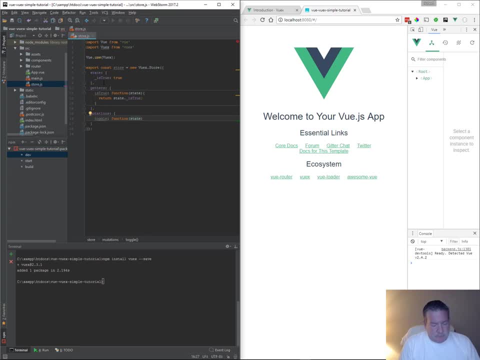 And then the dispatch does the same thing. And I'll put all that together here in just a second for you. 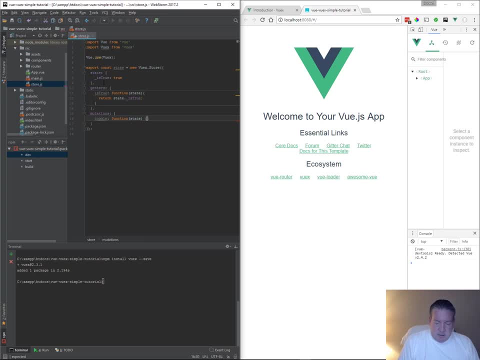 So we've got the function for toggle. And what we're going to want to do is simply take the state. Dot. Is true. Whoops. I thought that would finish for me if I spelled it right. 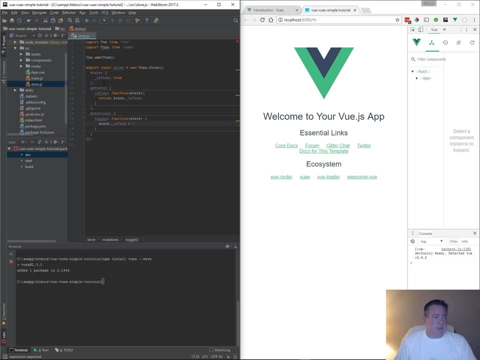 Is true equals not the state of is true. Which is, of course, because it's Boolean, we just turned it into false. All right. 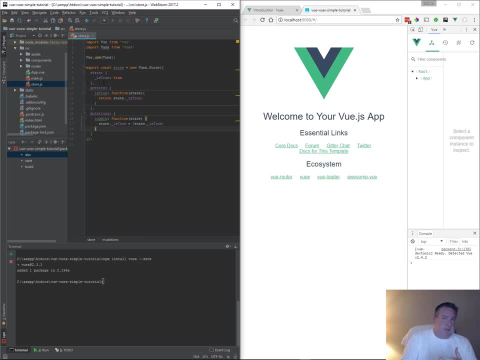 So now we've got our mutation. We've set the state. We've... Given ourselves the ability to go get it from another place called our getters. 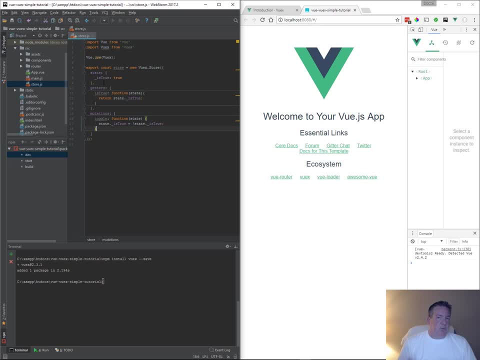 And we've created mutations. Mutations works synchronously. 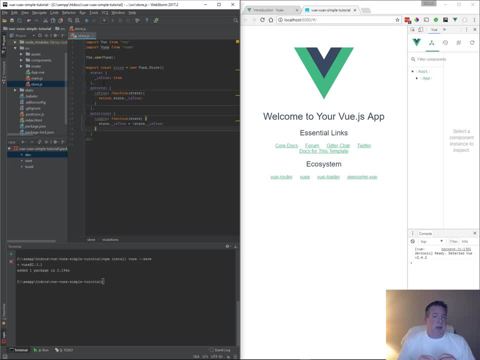 So if you need to do something like a call to an API, an HTTP call or something that, you know, it may take a little bit. Who knows? 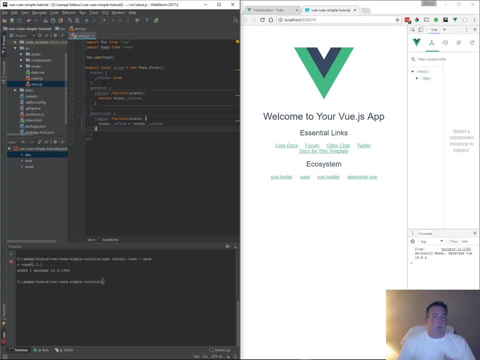 You can't use that as part of mutation. So we add a secondary layer and that's actions. And the... The actions allow us to do things asynchronously and then feed that to the synchronous nature of mutations. So in every case, your mutations and your actions work hand in hand. So we've got this state getters mutations and now we need to add an action to match the mutation. And the action is actually what the dispatcher calls, not the mutation. That's simply a pass through, a synchronous pass through. 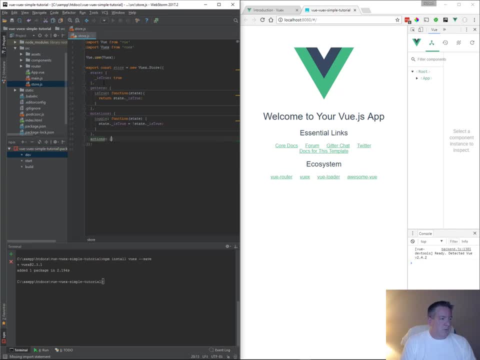 So we've got actions. And our action can be called the exact same thing or it can be different because maybe two different types of actions may still use the same mutation. They may just work on it first. 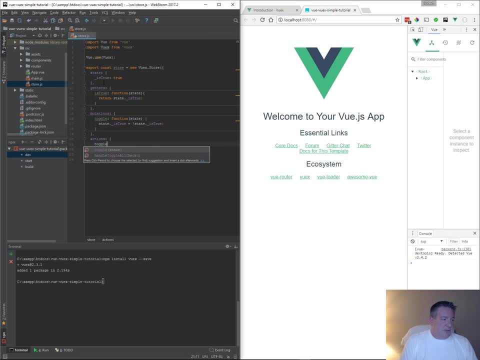 But let's go ahead and just in this particular case, we're going to do toggle because that's what we want to do. We want to toggle it, but we can't. We don't want to look at the mutation directly. We don't want to. We don't want to get into that. So let's do toggle and we're going to do it. 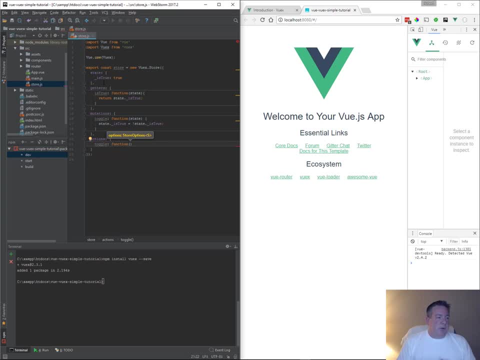 Function again, because everything's a function after that, and then we're going to pass the object of context. The context object is part of the store that allows us to access the state, the getters, the mutations, and I'm going to do it the long way first. So we're going to do context. 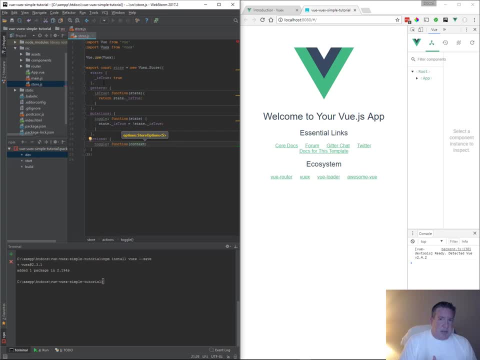 And if you needed to pass from a dispatcher, if you needed to get anything in there that was an argument so that you could operate on something within your mutation or even your action. You would hand it right here so you could, you know, you could pass in multiple arguments right here. But we're not going to because we're toggling and toggles just don't make arguments. We're just going to make it true or we're going to make it false, depending on what it is. OK, so we've got the toggle and all we're doing here is we're committing that to the mutation. So we use that context and that context is a fixed object. 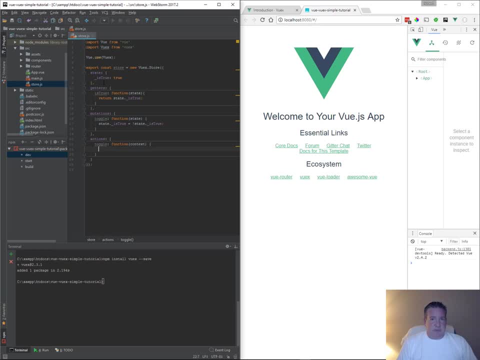 It's part of our store. You'll always have it in the actions. It's always going to sit there. 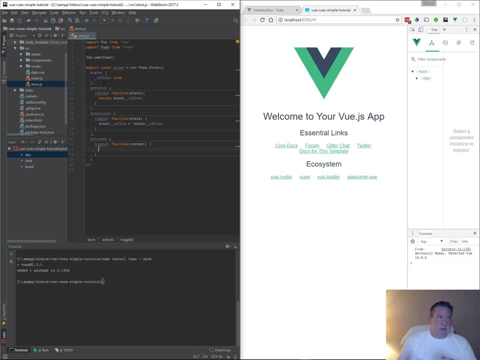 You can decentralize it. You can you can deconstruct it using ES215 2015 and deconstruct it and pull out because really what we want out of that particular object is it's called commit. I'm going to do a long hander and I'll show you. We do commit. Sorry, we use context dot commit. And then we're going to call the string. 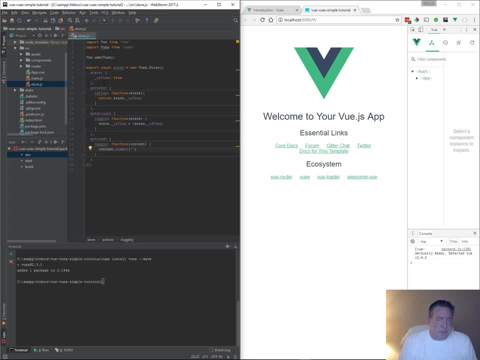 Of the name of the method in the mutation. So just toggle. 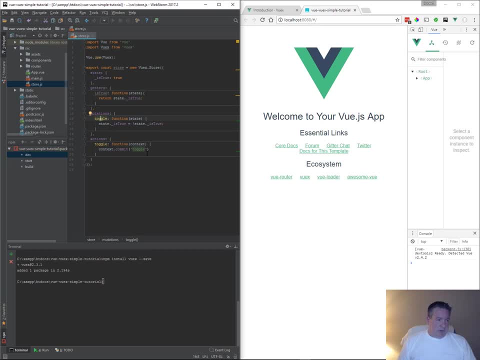 So what we're doing is we're this is calling this. You saw how it disconnected. 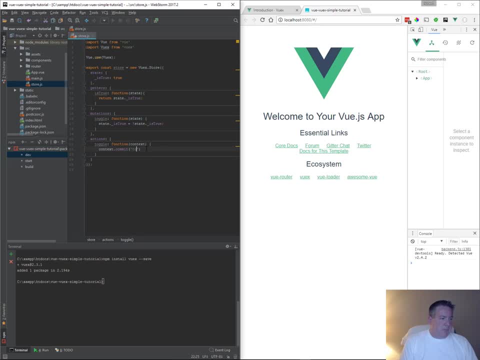 When that's disconnected, you'll see that that other one come up. So now we're connected, though. This one came up to we're not calling itself. We're calling this toggle in the mutations. And that's what that's what the context does. 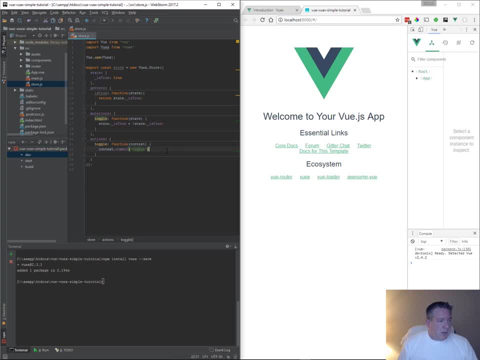 It links us to the mutations. And that and that's it. 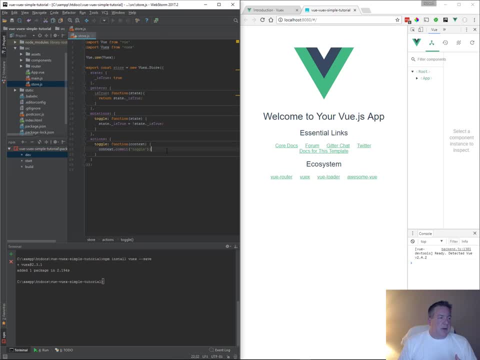 That's your entire store. And that's the entire control of this particular variable as far as toggling it, getting its return and setting its initial state. 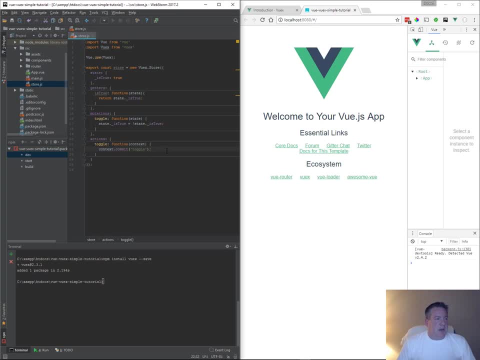 And I understand that that, you know, if you're looking at this, you're like, well, that's, you know, a lot of code for just for just what could be done in three lines. You know, you're going to initialize it, you're going to toggle it and you're going to get it back. But this creates an. Awful lot of extra protection. It creates time travel. 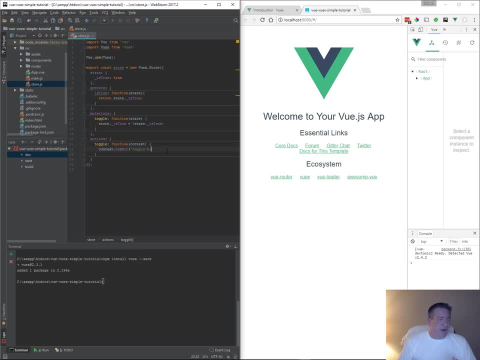 It creates a program of programming, time travel. It creates abstraction. It allows some encapsulation. 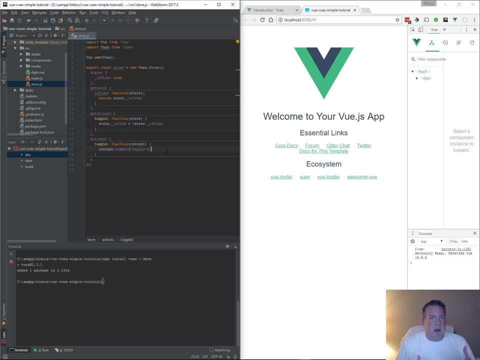 And if none of these things make sense to you, that's from a project that's from an object oriented paradigm. The idea is, is that it provides a lot of functionality and it still gets us to where we can abstract. Our store and use it with any component that we want to. And those won't conflict with each other. Not only can we do that, we can we can move the state back to a previous action or a previous event with no problem. 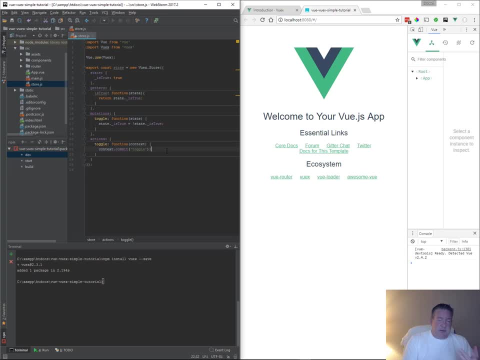 We want to move back to a previous event to see if we've got a bug or something like that. 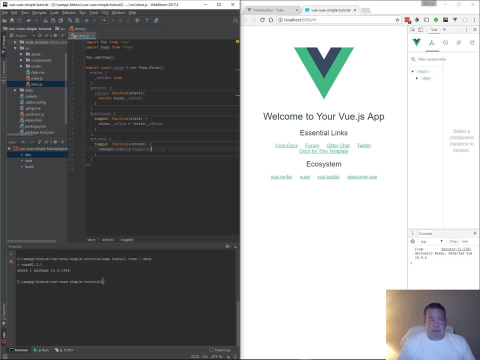 I'll show you how that works. The store allows us to do that, which you obviously can't do in three lines of code. 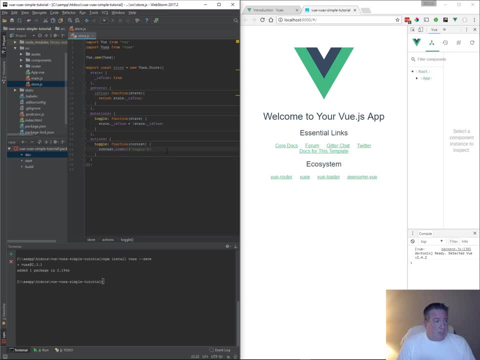 Just by doing the job script. But anyway, let's let's move on. 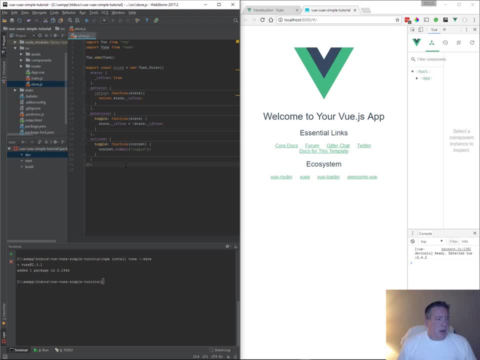 We're going to we're going to we've got ourselves a store and it's got the is true variable and every way that you need to to interact with that is true variable. So let's go ahead and save that. And we're going to inject that. We're going to add that or inject that into our application. And the way we do that is we look at main. In this particular case. You may name it differently. This is just how it's scaffold out with the web pack. And you may change that around. Who knows. 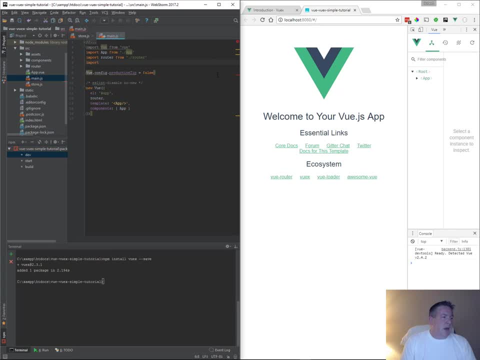 But we're going to bring that in and import. The store. Oops. 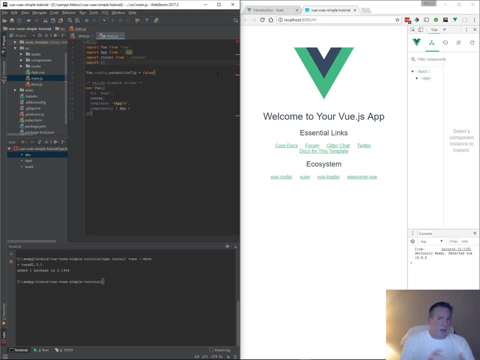 Oh, and because we we named it a constant in our in our module package, we need to actually pull using 2015. 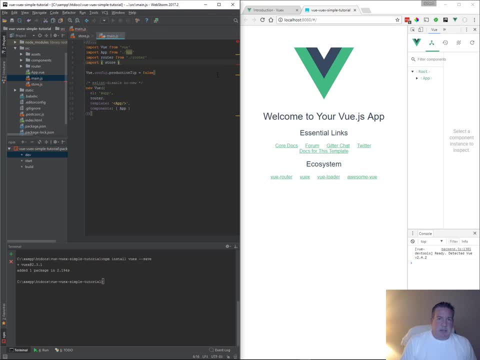 Deconstruction. We'd actually pull that out. So that's why I'm putting it in. And the the mustache handlebars, the brackets. 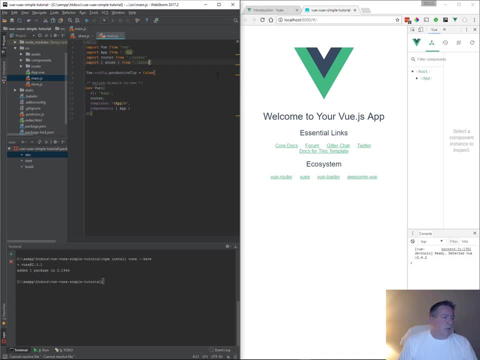 So we've got from store. OK, so so now we've we've brought the store into our main we've imported it and now that's it. Now we're in. Web store. 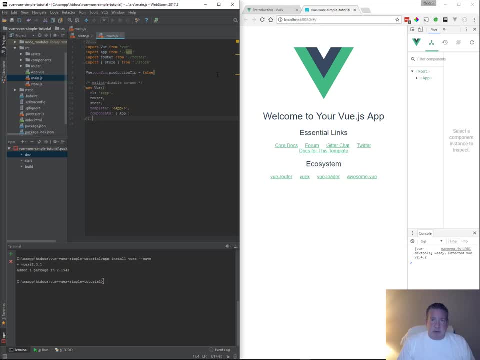 So obviously we haven't done anything to it. 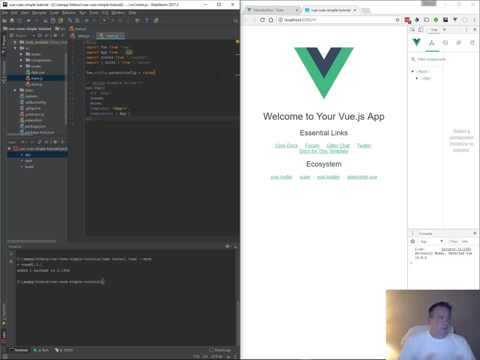 We haven't we haven't utilized. It in any fashion or form, but that's it. That's the store. 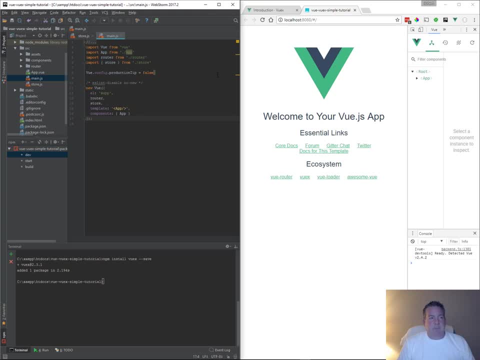 Now, if I were to do that without all the talking, instead of it taking 26 minutes, it would have taken three. And if you have that in a template somewhere, such as a text file or just or, you know, as a live template, it's 15 seconds and you're scaffold out for a store and you're ready to go. 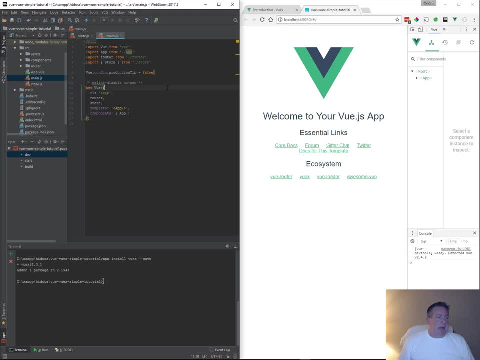 So let's go and use it. Let's let's see how easy it is to really be used. So you scaffold out your store. And we want to utilize it. 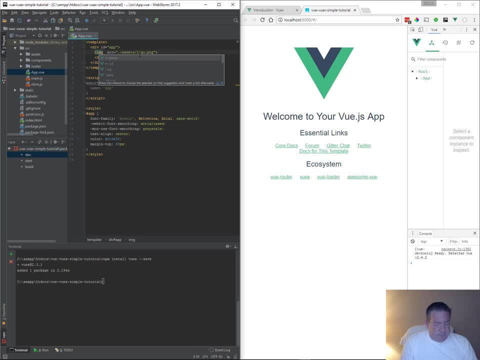 So let's put a VF. 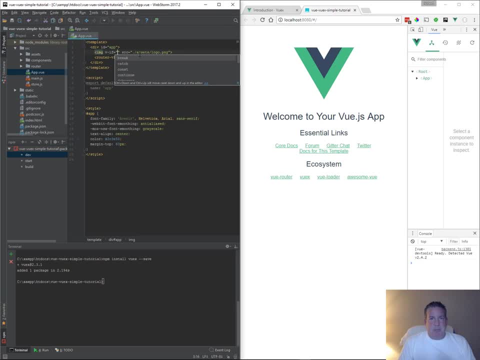 In our primary primary application, we're not even in the phone. We're just, you know, we're in a phone, but we're not even in a child component. 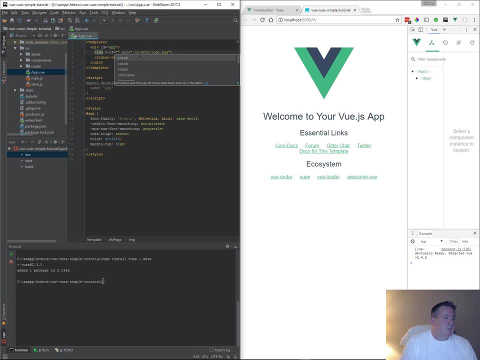 So if we do this, we're going to name it is true. 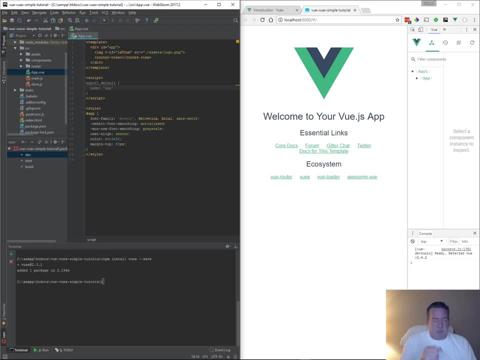 And it does. That has no bearing. That's completely local variable. 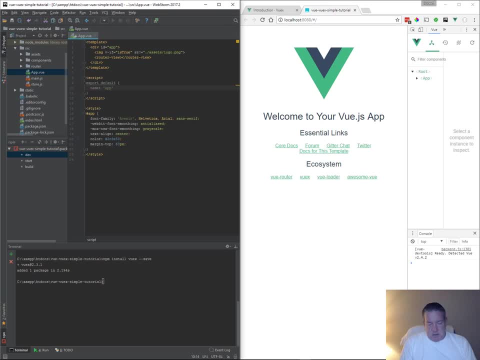 In this case, we're going to do it as a computed prop or a computed variable. So if you don't know what computed is, just go look at computed and watchers. 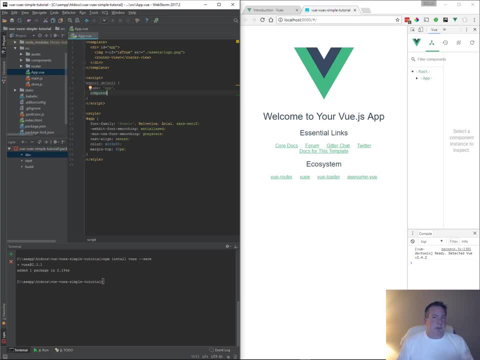 They're very similar. But what they do is they watch to see if the value is changed in any fashion. 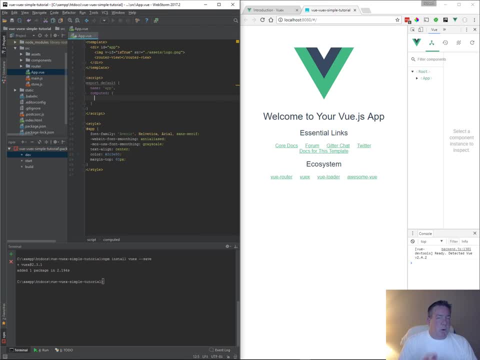 And we're going to want to watch this variable from the store, because if the store changes the variable, it's going to let everything know. That that that it needs to update the DOM accordingly. 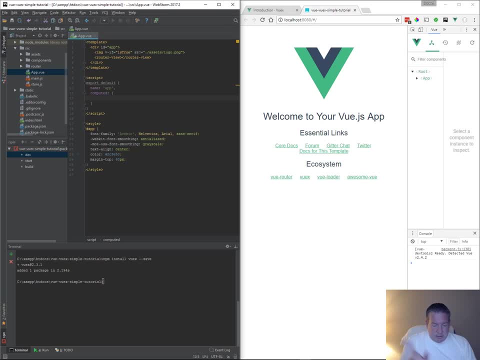 So we use computed here and we're going to we're going to bring in our is true as a function because it needs to tell us if it's, you know, as the function of whether it's true or false. So we do is true and we're going to do old style function. All right. 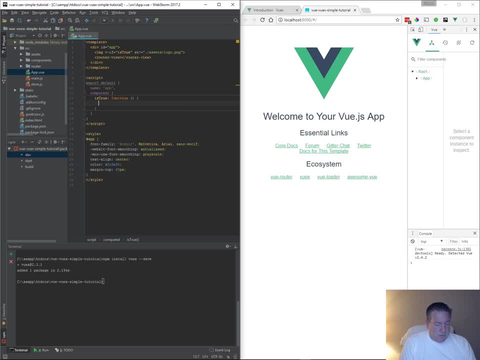 And from here, we want it to return. The store state. 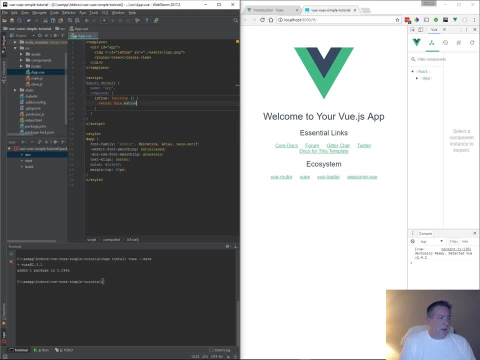 So we're going to do this dot store and we get the dollar sign store now from our store. It's now injected into the system. So every time you interact with the store outside of the store, so we're in app or main or one of our components down the list, you'll always start it off with, you know, the store. However, that needs to be this dot store. Or if you have to abstract this because you're in a, you know, tunnel. Into an Axios promise call, then you have to, you know, leads this into the into the it's a mess. Anyway, I love this anyway. So we're going to return this dot store dot getters because that's what we're calling. And we're going to return is true. And that's it. 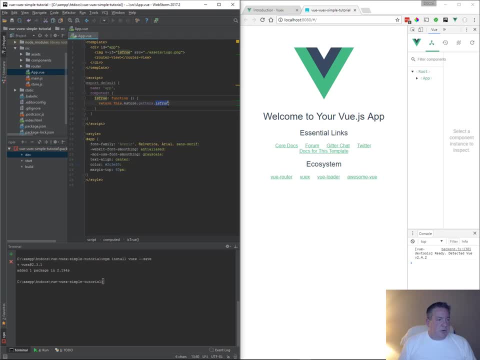 And this obviously this is true is the. Getter. Getter is true from our store. It is not. This is true. 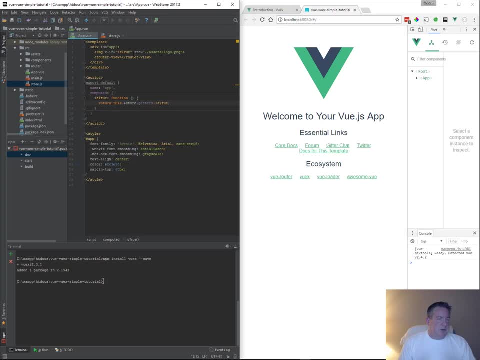 Funny to change that for any reason. And these become confusing. Let me know. 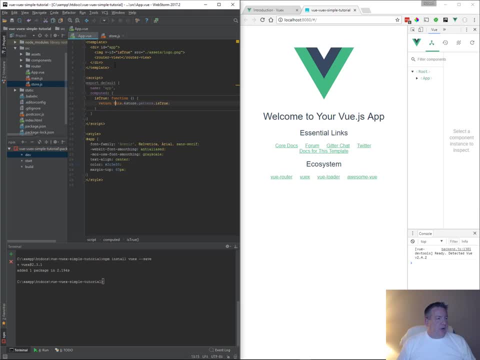 One of my problems I always thought was that that instructors would use the same variables over and over and over. And you're like, well, does that variable want that module or the other module? And is it important? Do they need to be the same? 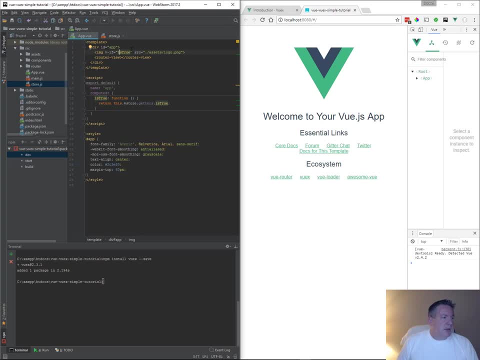 Anyway, this this variable. Is only associated with that variable. So we'll just leave that just like that is true one. 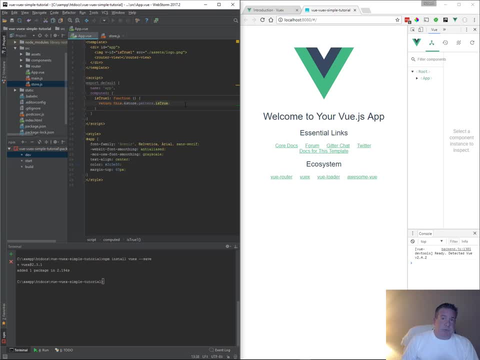 And of course, this very this variable right here is only associated with store. So now we have the abstraction that we need into the store and we're not pulling it in. 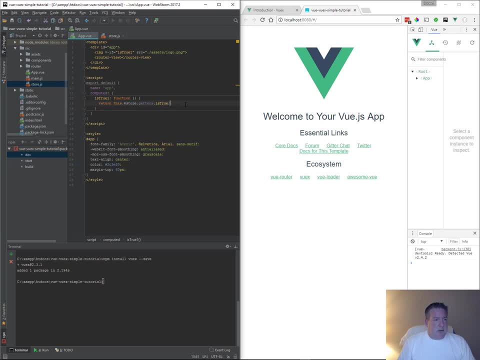 If I save this, you know, my my page is going to update and it did. But. But. 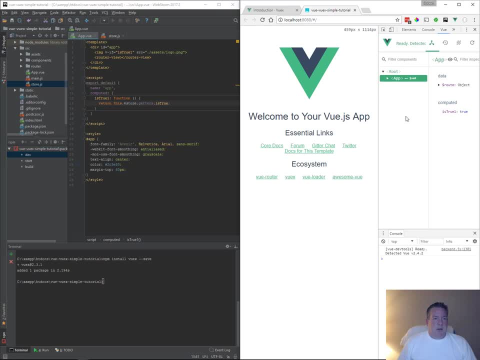 Is true one is true because our store is true. It's how we initiated our store. Our store came up and we turned underscore is true into true. So that's all propagating through now. And you can see it in our store. This is the state of our store. 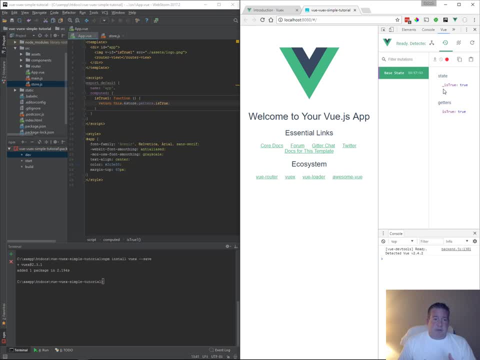 So is true is true. Is true from the getters is returning. It's true. 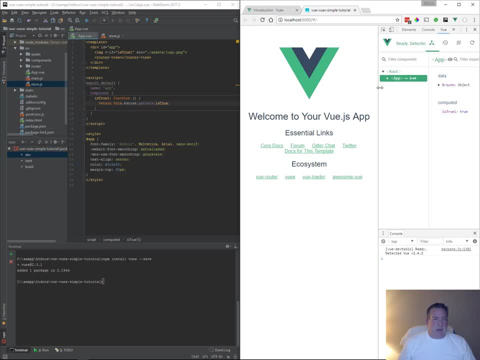 So now with our. With our little view inspector, we can look at the app and it's seeing the computed value. And our store time travel system is kind of seeing that currently everything is true. So it's applied. 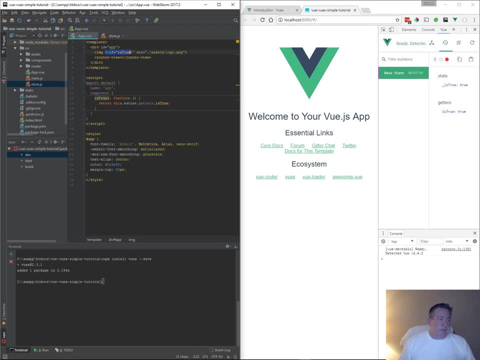 If that was false, our image would just disappear right here because if would be false. So let's trigger that by adding a button. 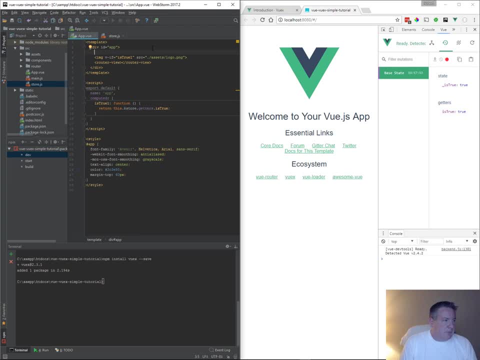 Let's do just a simple button. And we'll do button. 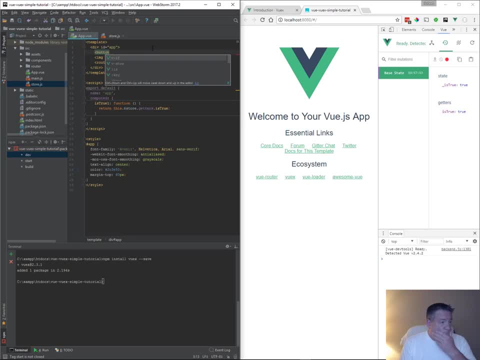 And we'll do I do it long hand or shorthand. We'll just do shorthand. 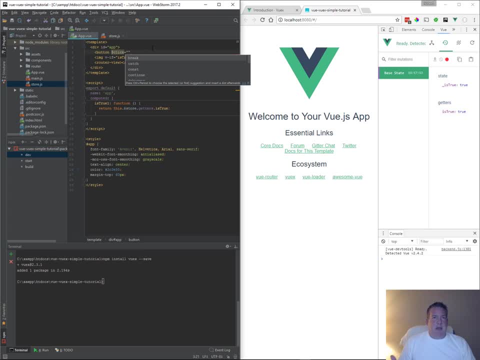 Shorthand event for the button you do at click or you can do the on colon click and we'll just give it a toggle me. I just call it toggle. But again, that would be my style of coding and that would be a problem for some people. are watching this and going well does that toggle match another toggle that's in the store toggle 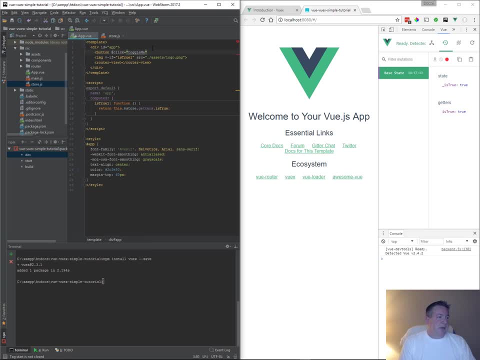 not at all this is completely local so we're just going to say toggle me um and then you know we'll call it toggle and let's see where that button shows up we're going to get some errors down there because we don't have a toggle me function uh let's see vr area but we just want to make sure that button doesn't jump around every time i eliminate the picture so we put it above it would 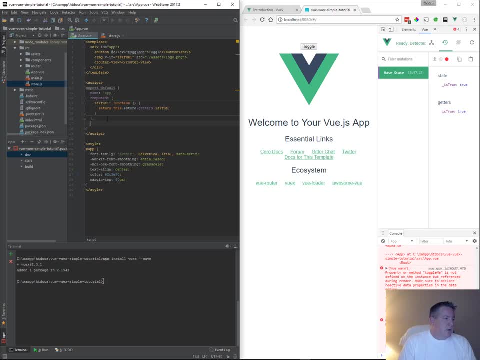 be fine um all right so we're gonna now we need a method for that so you know this is this is standard old old view uh and we're gonna name it toggle me 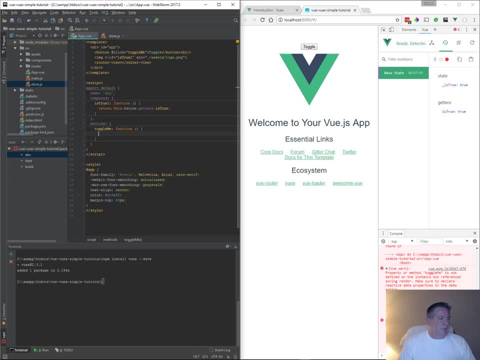 all right um and then in the toggle me you know we can pass an event or not my in in webstorm and 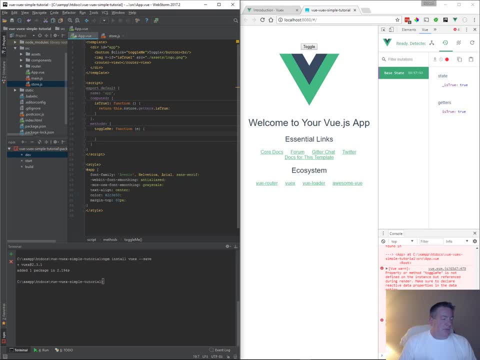 php storm one of the reasons i don't just i automatically pass the event is because if i don't use it it gives me a little gray under squiggly sign and says hey you're not using this this variable do you really need it uh we'll go ahead and leave it there for now but sometimes you need it sometimes you don't uh okay so uh 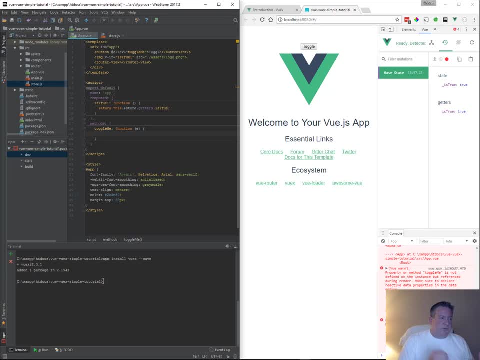 toggle me is gonna now now this is it we're gonna dispatch to the store and say hey store do what you need to do to this variable and then transmit that everywhere so we're going to use the store so 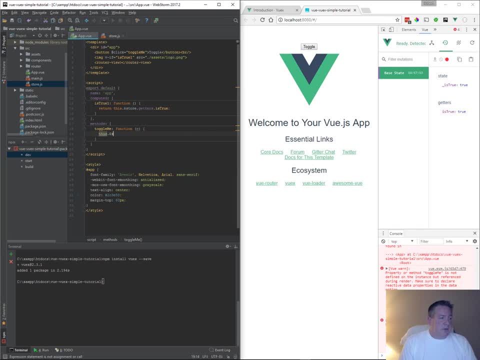 uh my hands are in the wrong place this dot uh store and not thus goodness gracious right not store um 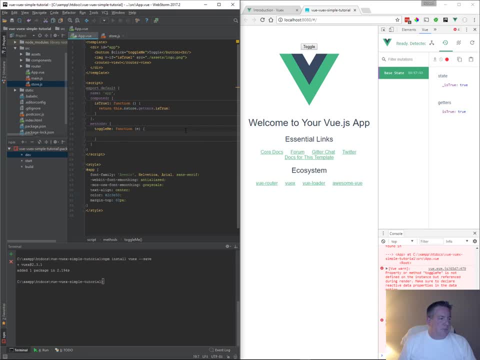 now i've got something else messing here let's make sure my e's not messing that up this dot store dot dispatch 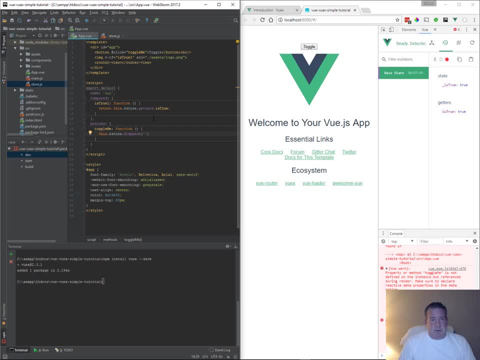 remember that dispatch and then we're going to dispatch whatever uh whatever the the method is uh action that we're going to need so in our store we're looking for this this uh toggle action we're looking at this one not the mutations uh so in our app we're gonna dispatch toggle so basically what we're gonna what we're gonna see is that um 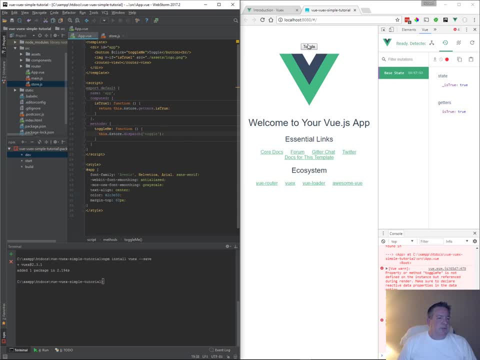 let's go ahead and save all that when we when we hit the toggle the image will disappear and that's simply by the fact that we hit the toggle that calls the store's action from the store's action we go from action to mutation it mutates the is true to the opposite of whatever is true is the time which is currently true which will make it false then from there we've mutated that to false and then the getters triggered by the computer property will return false right so we've kind of got this round robin we dispatch to the action the action goes to mutation mutation alters the state and the computer properties pull from the getters and and we end up right back where we are and this is true one which is pulling the getter is true will change values and because it's watching it through the computed uh property um it will change uh and the dom will take care of the rest the virtual dom and the real dom obviously and so we hit toggle and it's gone and we hit toggle and it's back uh and that's the store that's not using props and emits that's not uh if we had another uh well let's let's put let's put use the store and same variables that we need and let's put it on a secondary component because that's the important part right secondary component um so we look at our components 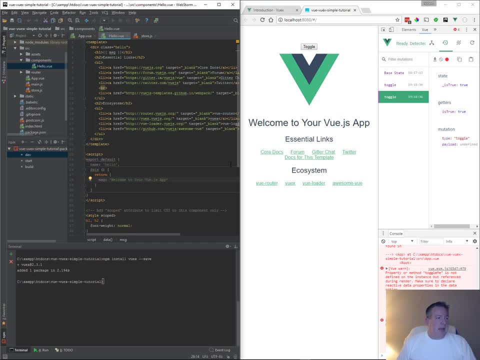 and we look at hello view uh yeah and and let's just make the whole thing disappear with the same toggle button from that's that's altering the store um we'll just add v show 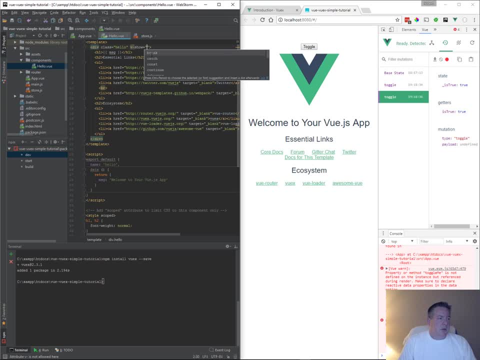 uh and we'll do it the same thing we'll do is true too so that we don't keep crossing over variables and nobody thinks that one variable needs to be associated with the other one this one is completely local to this component 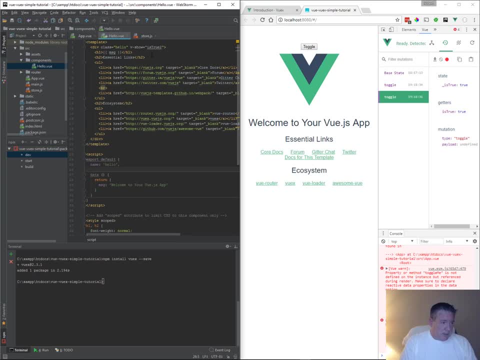 okay so again computed property computed and then same thing we're going to do the whole uh uh is true to this time so we can match this this one matches it's going to be a function um we're not passing the event and uh so from here 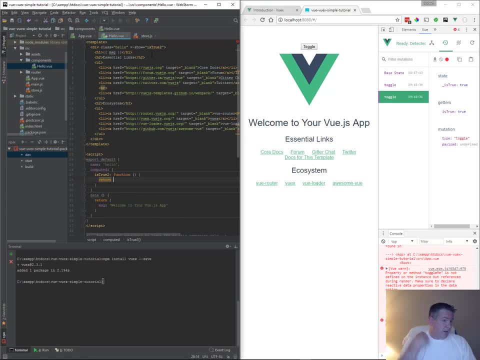 dot store dot getters dot is true now that is true is the one that's in the store so you don't want to confuse that with the is true too that is local 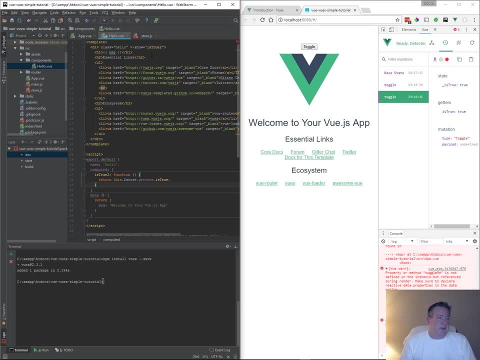 okay so now you've you've got that that's it you're not dispatching anything because you're not changing anything uh that's happening in the previous or other component uh but this one is going to obey the laws of the store um with just that so now if i'm going to do this and i'm going to 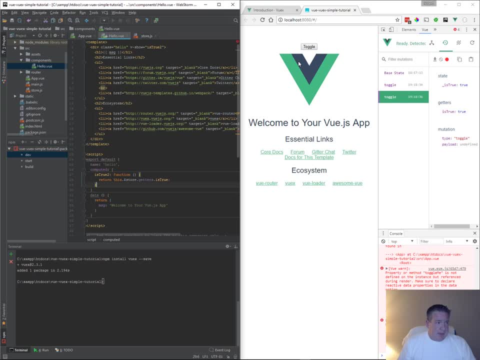 hit toggle and it goes to false i'm going to lose my image and i'm going to lose the entire the entire component uh visibility because show is going to turn into false and the only thing that's going to be left is a button which i get to toggle again and turn it right back on so now we've got off whoops 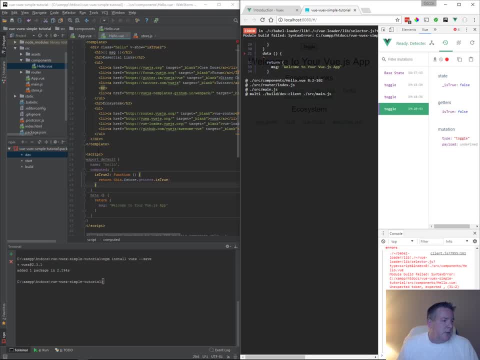 oh always leave your bugs in so they see that you're not infallible okay so i forgot my comma right there 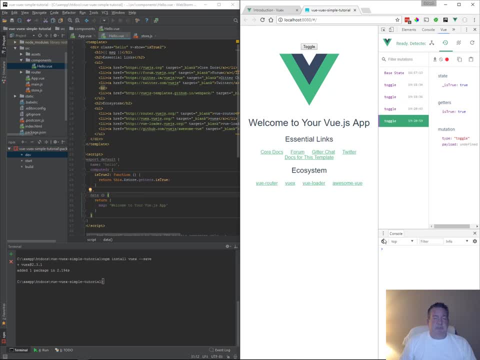 um let's bring that back lost its poofness anyway uh yeah so toggle gets rid of both brings it back in but notice on the right 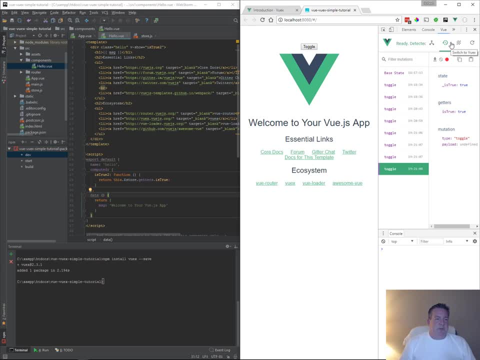 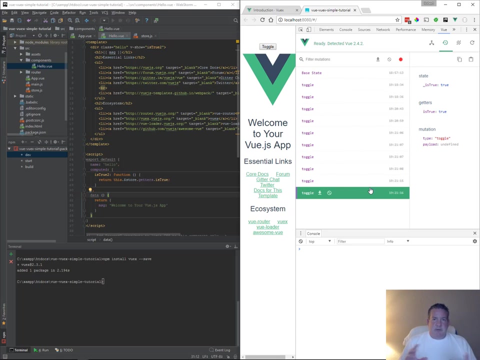 hand side now see you've got your store and so if you didn't understand what time travel was you're seeing it now every single time i do it they it stores the state of how it was previously and you can go back through this and you can you can no matter what you do you can go back through this what's happening uh you know we're not doing simple toggle maybe we're doing some calls and some more much more complex uh much more complex uh mutations and we need to find out where a particular mutation may have caused a bug you can you can time travel as it says to the state um you can revert to this mutation and eliminate all other other mutations past that um 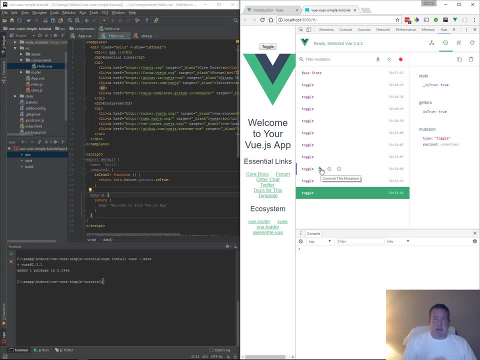 and of course you can commit that and that would commit it as a bug the base mutation but if i want to time travel back to this or this or this it's as simple as that and that's what the store allows you to do that would obviously be real problematic if uh if you're just doing your three lines of of you know let this equal true uh a real quick uh inline 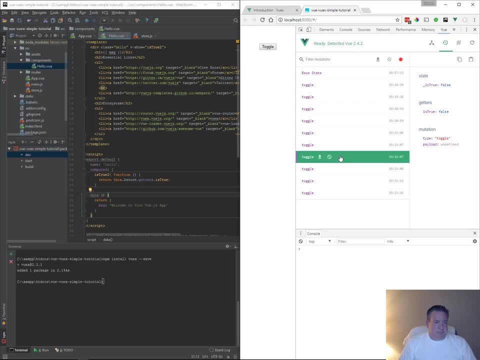 function for toggling and then and then uh uh i i don't know now whatever the three lines were i said earlier 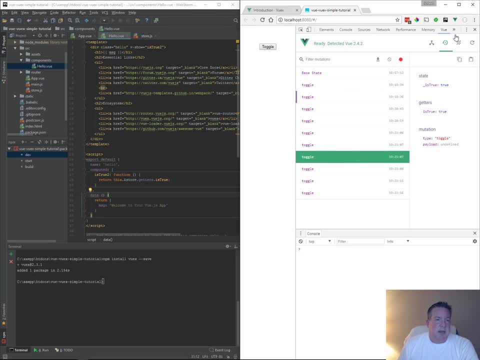 anyway so so that's it uh you've got your store state of course your events um no events i'm not sure i have to look into that why why we're not seeing any events that i have to see what that component's actually looking for in events um but but we've got a root application you know you can see that we've we've got the is true one which is local to the app component we've got the whole store here which is showing us 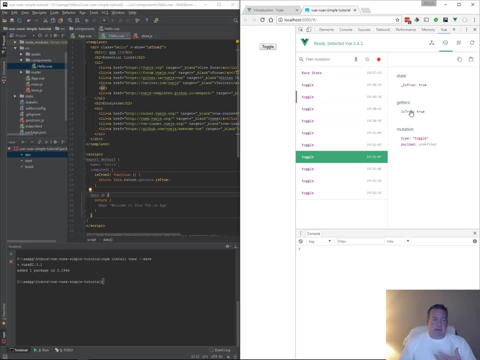 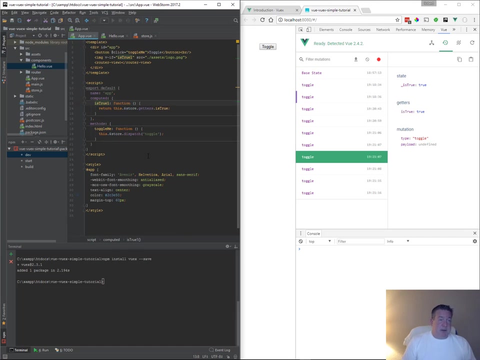 that the state is set to true the getter is set to true uh because of the state and the mutation uh type of toggle which doesn't have a payload remember we didn't we we'd sort of let me show you that real quick if i wanted to look at app view and i wanted to dispatch something with 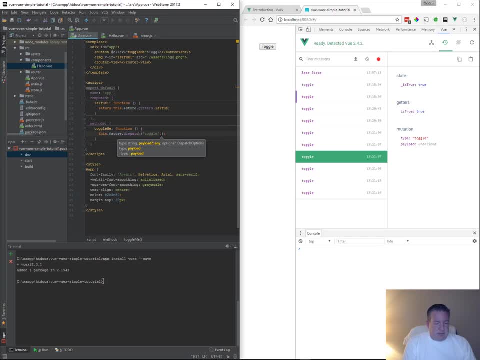 the payload all i'm doing is adding the payload so that i can i can add the bull i can add true 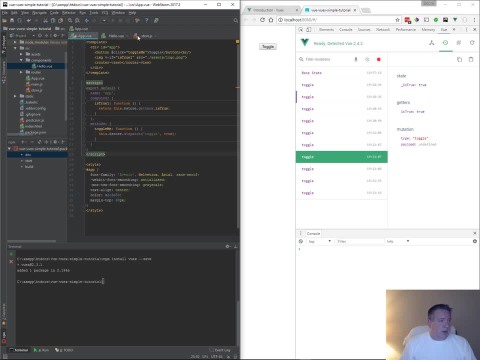 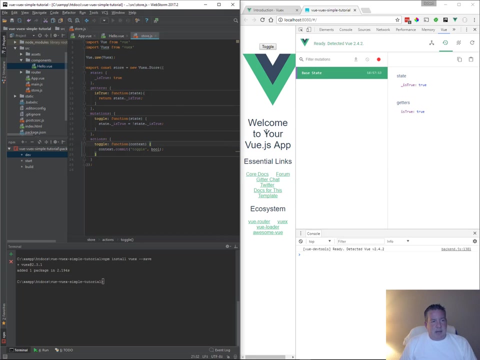 right uh and of course this doesn't care because we're not going to use it uh and we're going to go to the store and we can say hey uh in my actions i'm looking for a bull i'm looking for a variable i'm just going to call it bull um and it it just doesn't it doesn't care uh 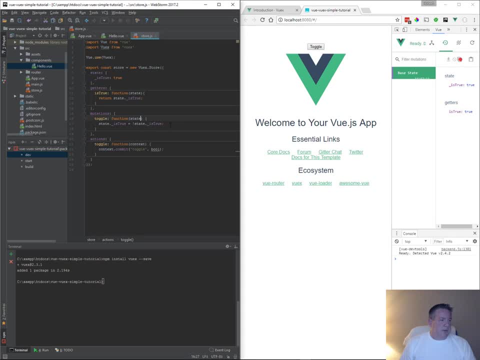 because we're not using it and then you know if i want to toggle the google down um you know 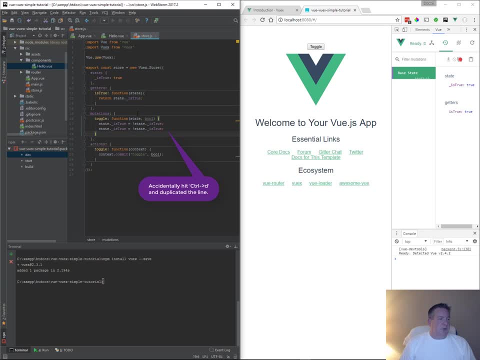 then i can bring it in from from my context commit to the the uh sorry there you go so now we've got all three of them working in action we just pitch it we dispatch it to pitch it just dispatch it it it comes into the toggle 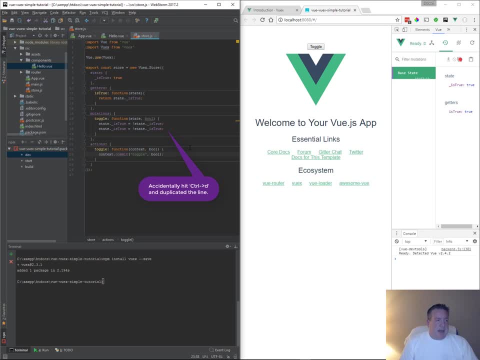 function and the actions the actions then context commit it out uh into the toggle in mutations uh target mutations brings it in and you know we do with it whatever we want to 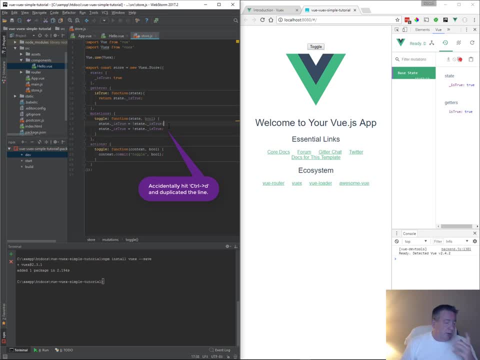 you know who knows uh in this particular case we're just doing toggling so uh the rule just doesn't make any sense anyway uh i hope that was helpful uh it was a little bit longer than i expected um but i hope it was thorough and i hope i hope that everything made sense um if you have 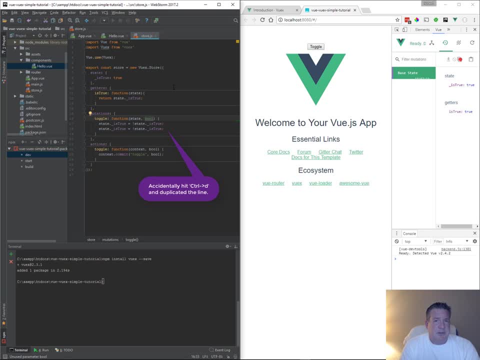 any questions or you need any anything further explained you didn't like anything i talk a lot and i talk fast the beauty of video is you can stop it at any given time and just look at stuff um you can even slow it down 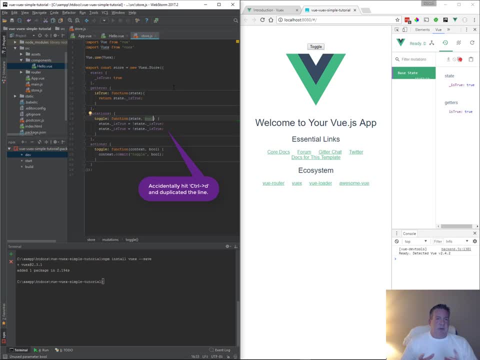 but but if you have any questions you need to have any anything else with the the basic implementation that's the beauty of this this system is is just throw in the view x 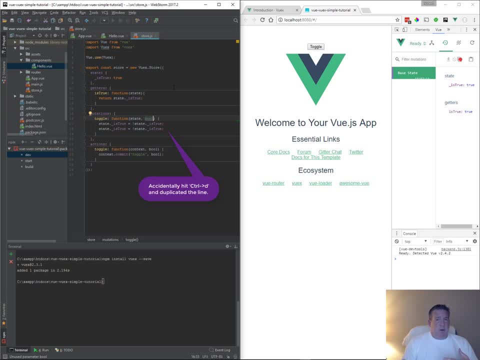 into your view it should really come into the cli i don't know you know they give you the router and they and they and they scaffold out the router but they don't give you view x i don't 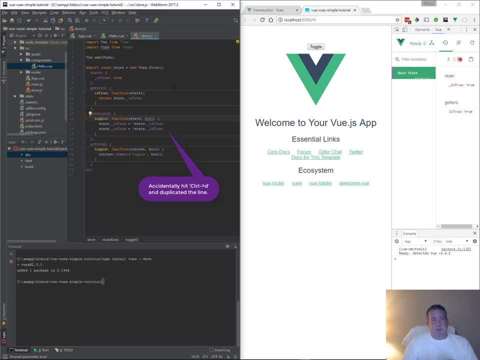 know why because i can't imagine building almost any application without having a store now when i when i didn't understand it sure as i avoided it eat the frog um but but 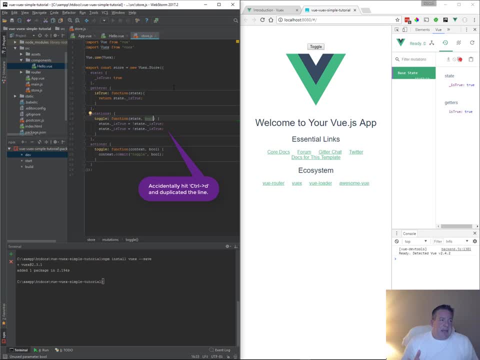 uh but now that i understand how the store works i i can't i can't live without it and i wouldn't want to try and write props and emit uh events and and and put them into a parent to bring them